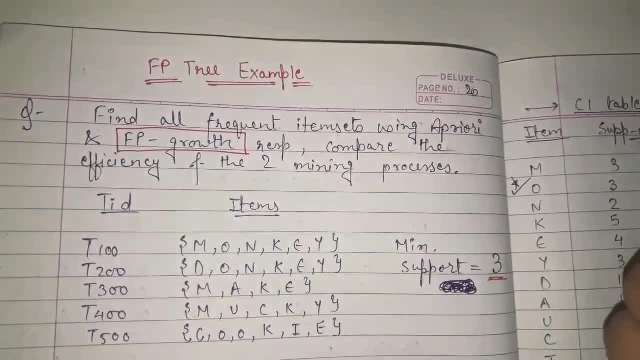 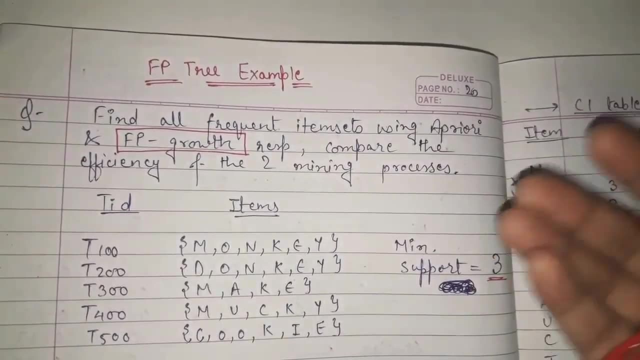 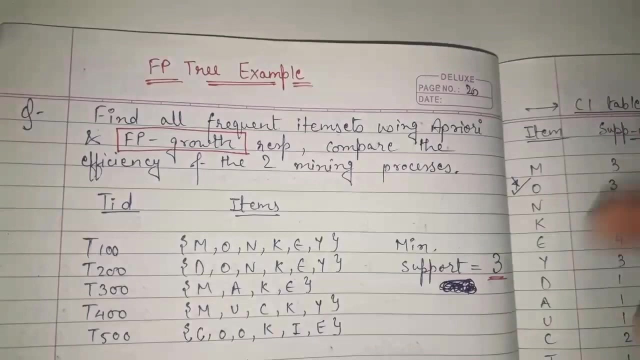 Now we have to solve this. We have to make a FPTree and, based on the FPTree, we will make a table and, based on the table, we will take the decision that what is the frequent pattern we are getting here And in this video we will see, with the help of this example, the whole procedure in detail. 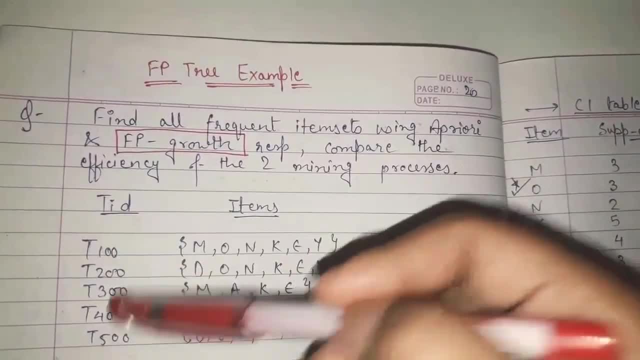 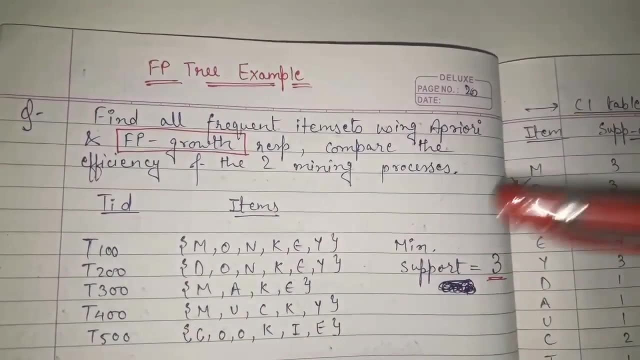 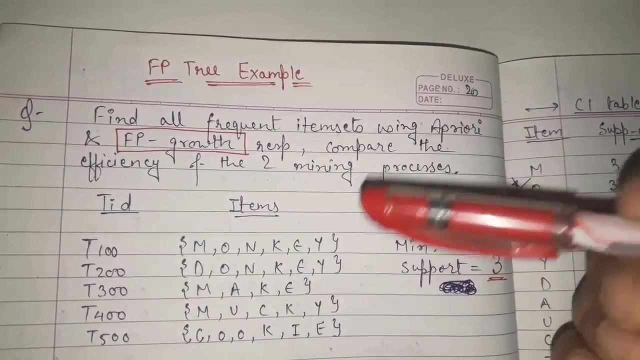 Fine, Okay, So this is the question given to us. Five transactions are given- T100, T200, up to T500- and their respective items are given Now in the example of a priori also, I have taken the same example and I have shown you how to apply a priori algorithm in that. in that, what was the frequent item set? we have got O K E. 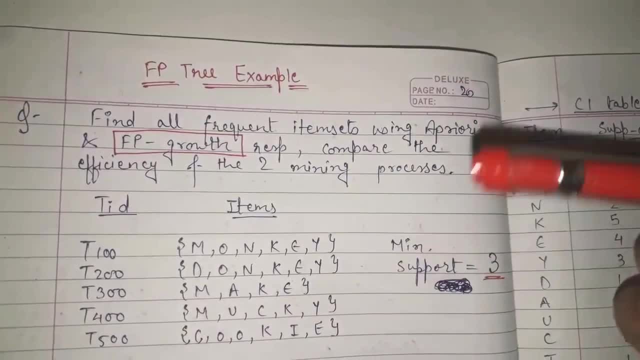 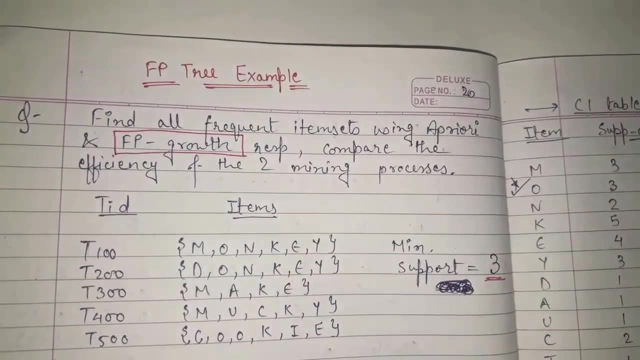 Fine, O, K and E. These were the three frequent item sets that we got in case of a priori. Now let's apply FPTree or FP growth algorithm in this and let's see what we are getting as the frequent item pattern. 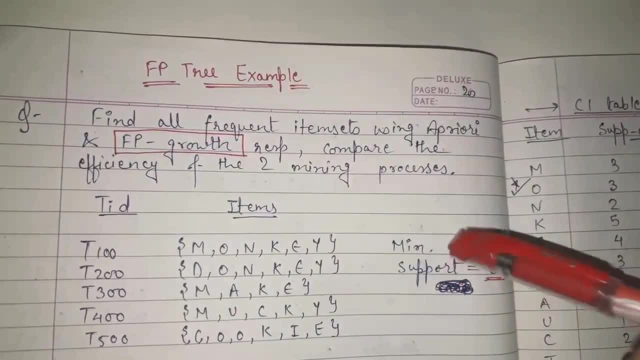 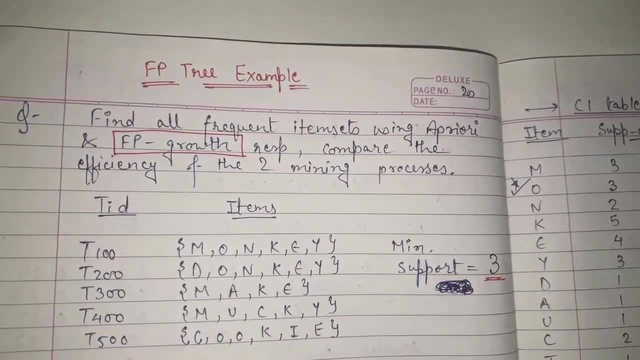 Fine, So this is a transaction ID is given, items given and also minimum support count is given to us. That is three. Fine, These things are given. Now what is the first task that we need to do in FP growth? similar to a priori algorithm. 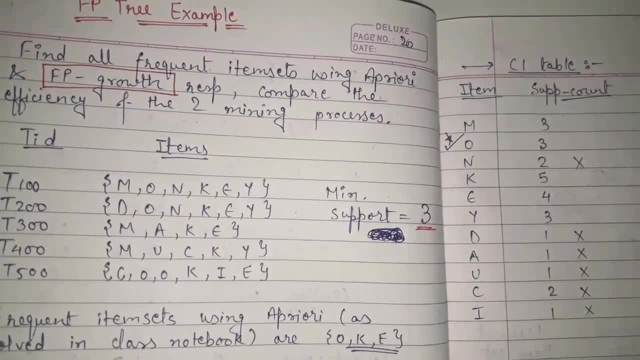 First of all, we have to make C1 table and L1 table. This first task, or the first step, is similar in both. In a priori also, we used to make C1 table and L1.. Here also we will be making C1 table and L1 table. 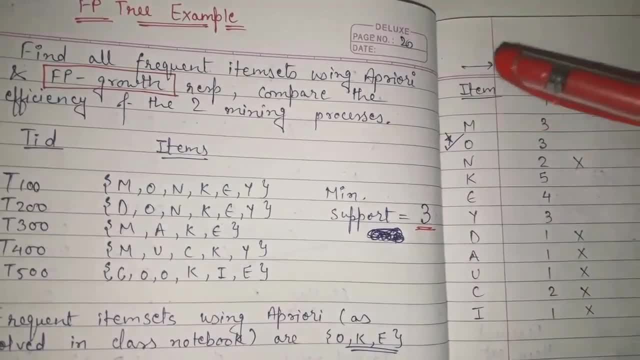 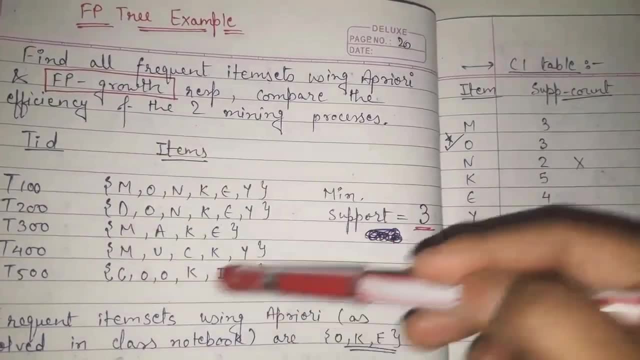 Now let's see what is C1 table. In C1 table there will be two columns, that is, item and support count. What will come in the item? In item? whatever items are given to us, these all are the items given to us right in our question. 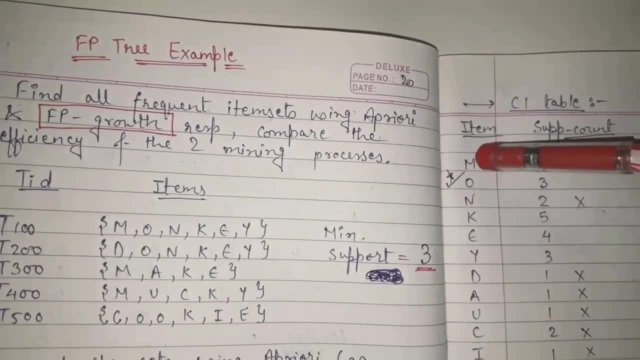 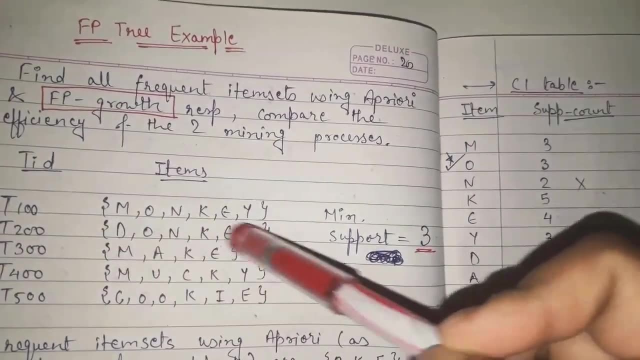 Now all the items we will be writing down, or noting down, all the items, unique items here, Fine, For example, see M O N K E Y. all are coming For the first time, so M O N K E Y, we will write down. 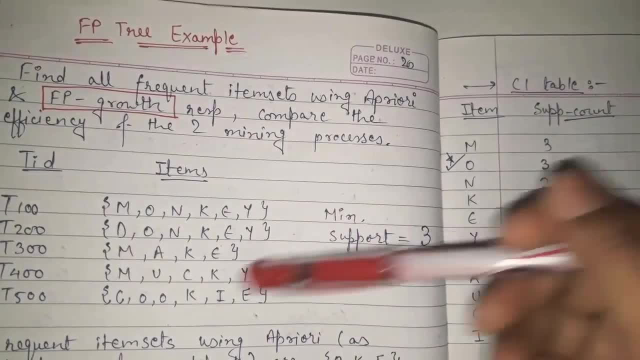 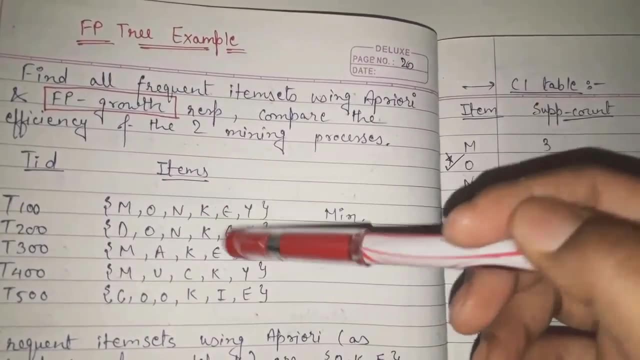 D. Now D is coming for the first time, so we will write D Now. O, N, K, E, Y is being repeated. It is already here, so we will not write that. So, in short, from all the given items, we will note down all the unique items here. 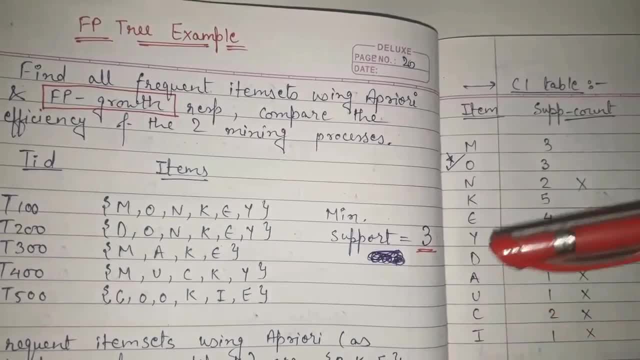 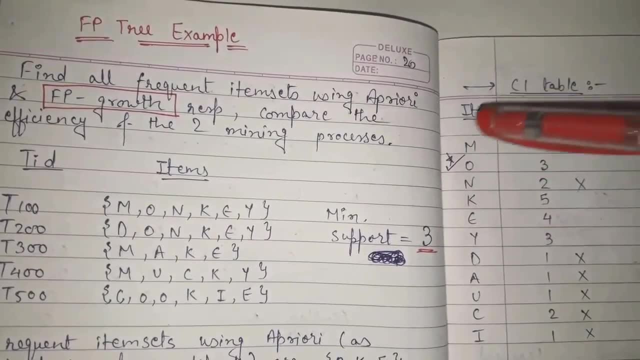 Fine, So in the item column we will first note down all the unique items. Now in the support count. what we will do, Whatever item is, we will count that in how many tries. So in the first transaction this item is present We will write down that count or that frequency here. 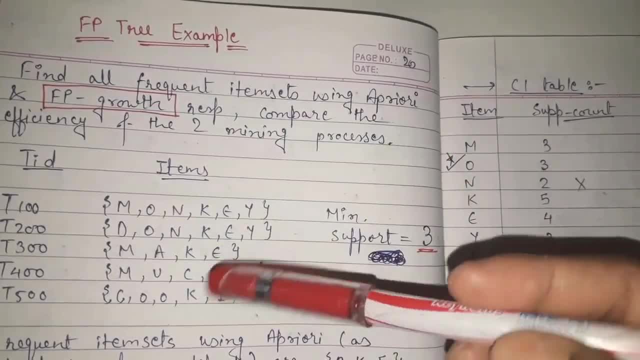 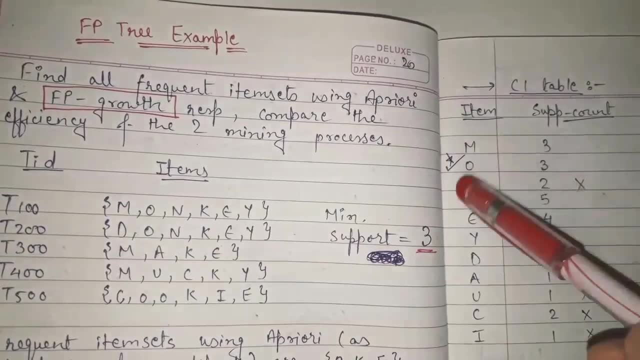 For example, first of all we are having M. So if I count M here, M is coming here 1,, 2 and 3.. Fine, So M is coming 3 times in 3 transactions, So we will write 3.. 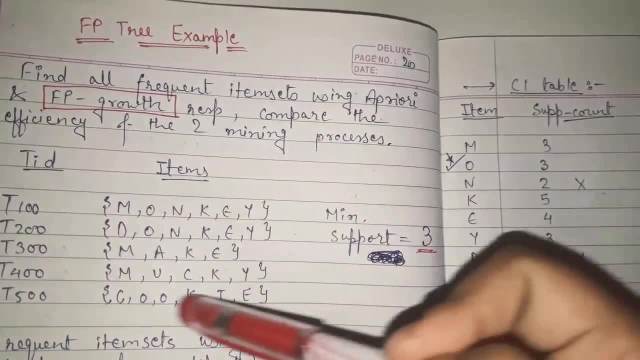 Then we are having O, So that O 1, 2 and yes, see, this is an important point, that if you see, in the 5th transaction we are having 2 Os, But here we will not count it as 2.. 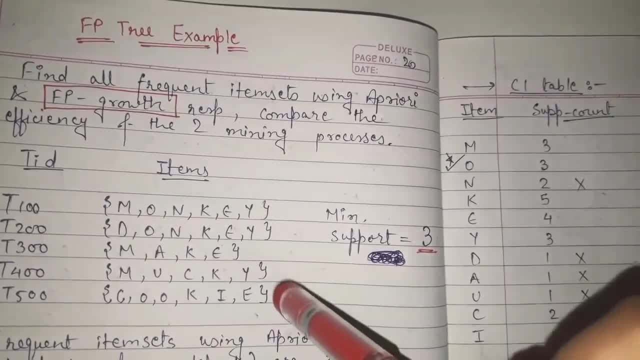 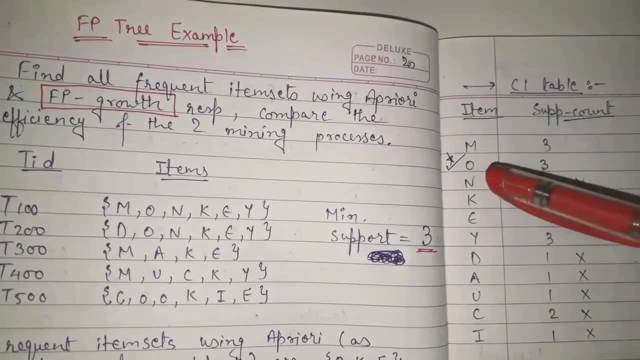 We will count it as 1.. We will count it as only 1 because in frequency or support count. what we want to see is that in how many transactions this item is present. So if we just count about the transactions 1,, 2 and 3.. 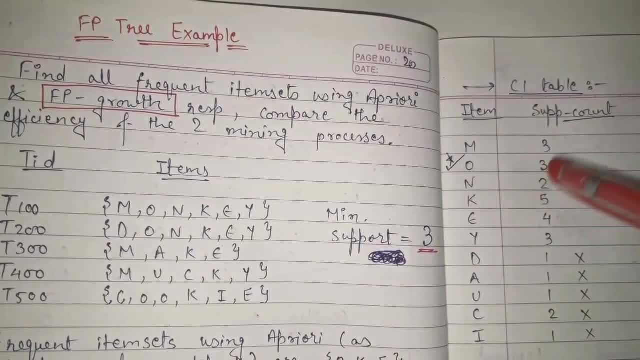 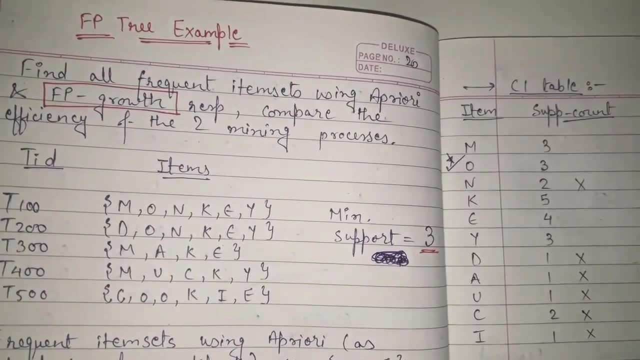 So there are 3 transactions in which O is there, So we will write 3.. Got it? That means what, if any? if in any transaction any item set is repeated twice tries or more than 1 times, Then also we have to count it as 1 only. 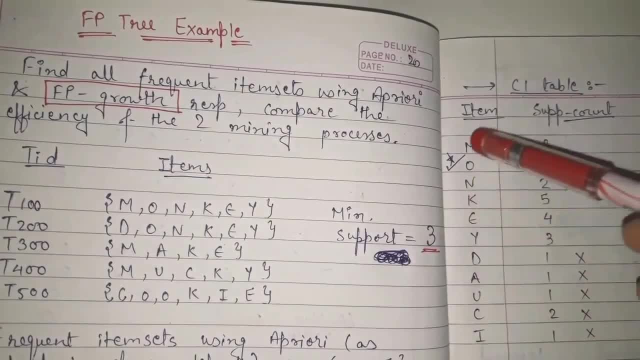 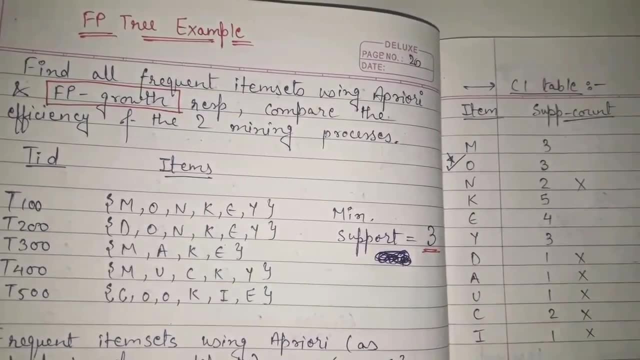 Fine, So, similarly, we will count The frequencies of all the item sets and then we will write it down in support count column. Fine, So this is what our C1 table is Now. the next task, or the second step, is to make the L1 table. 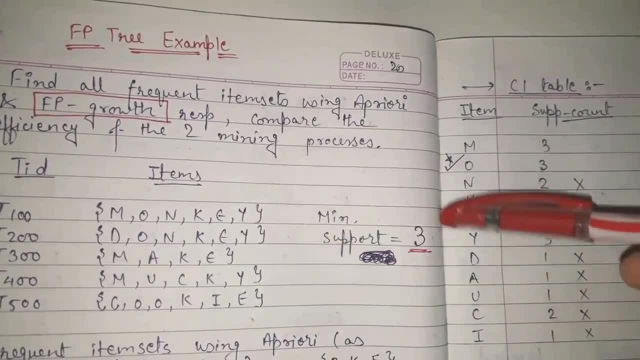 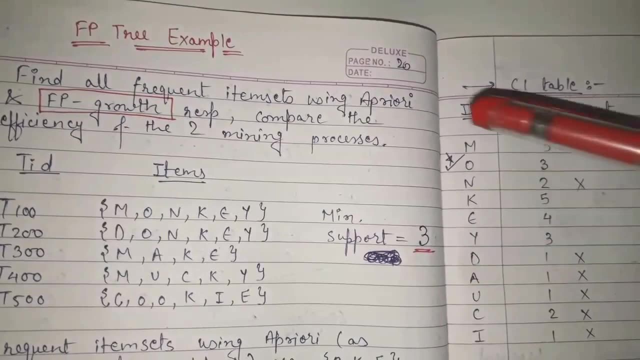 Now what do we mean by L1 table? See in the question we are given minimum support count equal to 3.. Now what do we mean by minimum support count? that whenever any item is having support count less than 3. Then it is useless. 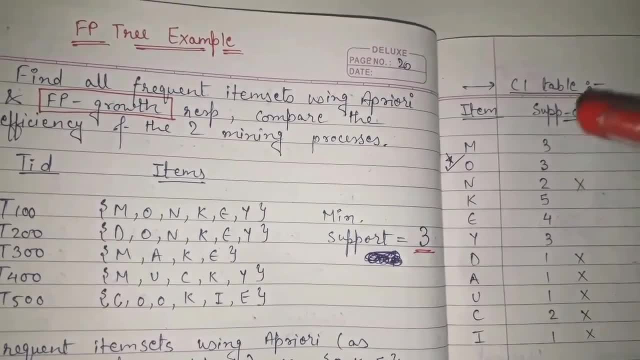 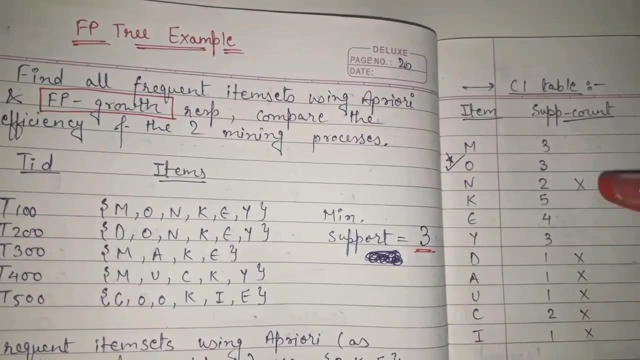 It will not come in our frequent item set. Fine, So what happens in L1 table? In L1 table we will select only those items from C1 table that are having support count as minimum 3.. That means the support count should be 3 or greater than 3.. 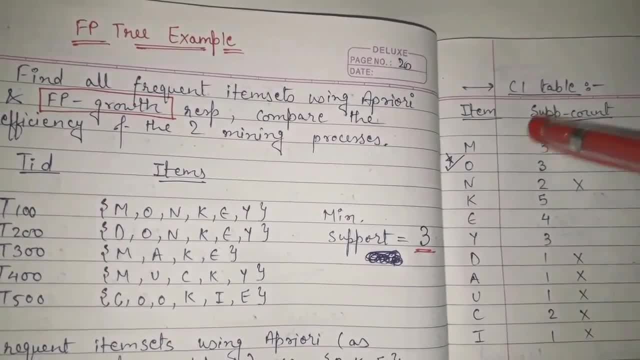 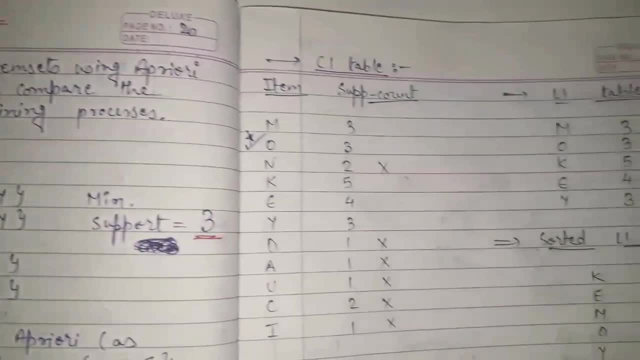 That means for the items that are having support count less than 3.. We will simply cancel them out, See 1, 2. we will simply cancel them out And wherever our support count is 3.. Or more than 3, we will write them down in L1 table. 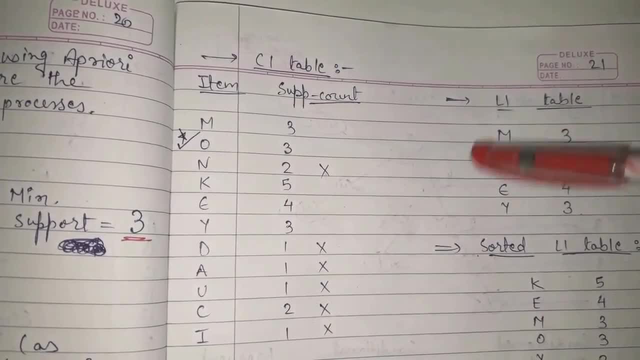 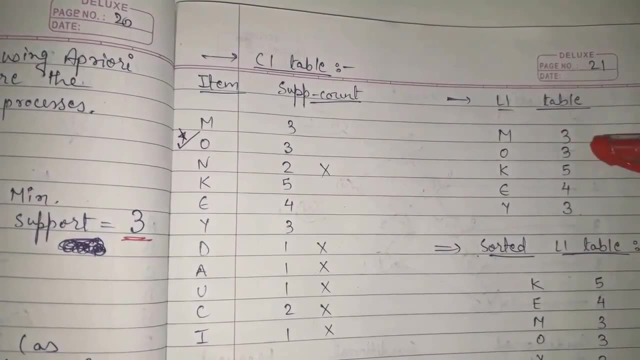 Got it. So L1 table will only consist of the items that are having frequency or support count at least 3.. Fine, We have done that, Okay. Now, after making L1 table, our next task is to make sorted L1 table. 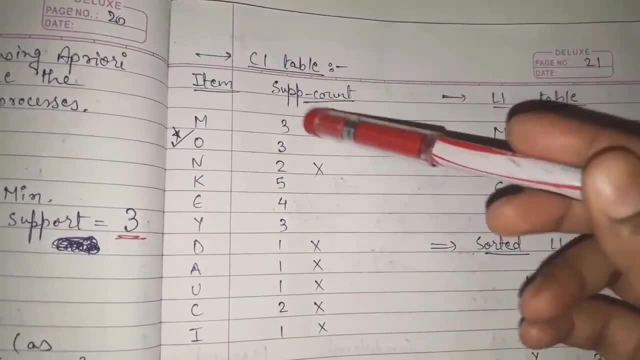 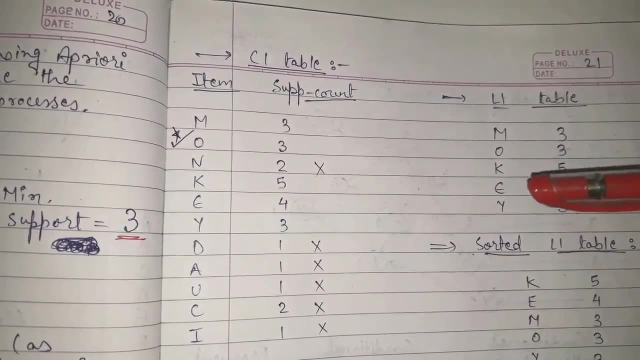 So here, what we want to do is see This C1 table, making this C1 table and making this L1 table. you must be knowing, Because this task we are doing in a priori. also Now, after this step, the further steps are new. 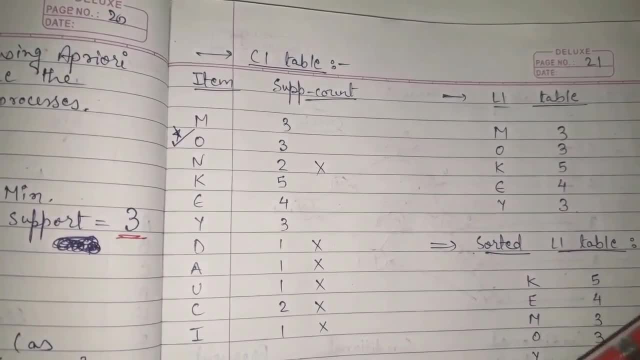 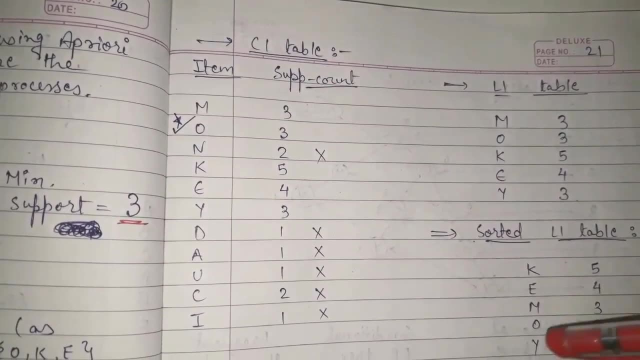 Further steps are new for FP3 algorithm, Because those things we were not doing in a priori. Fine, So upto here is okay. Now see the next step, what we are doing In this case, in case of FP3 algorithm, we want sorted data for L1 table. 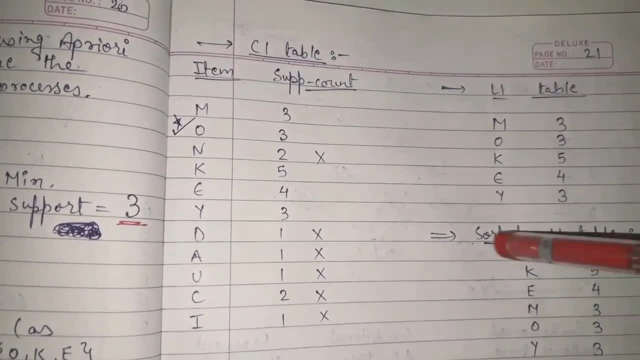 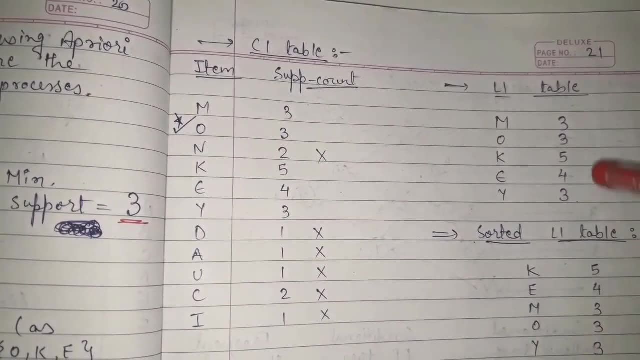 So after finding the L1 table, we will just make sorted L1 table Where we will sort this frequencies or support count in decreasing order. Fine, So these 5 numbers, We have sorted them in decreasing order, that is 5, 4, 3, 3, 3.. 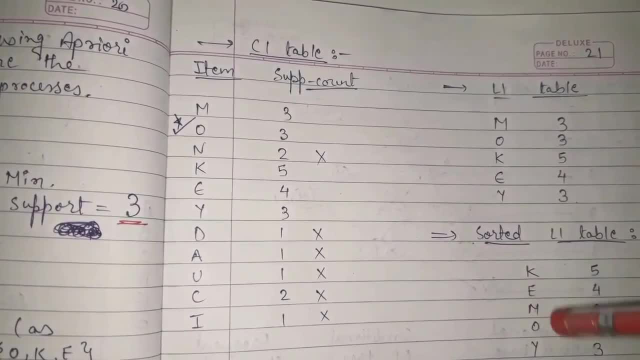 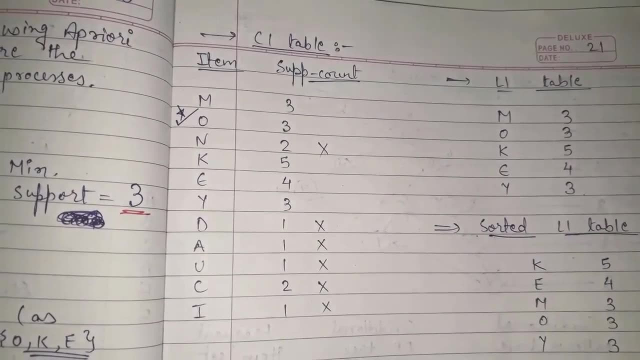 So 5 means K will come first, E will come second, and like that we will draw our sorted L1 table. Fine, Okay, It is easy. Now, after making sorted L1 table, what we will do is What we will do is: 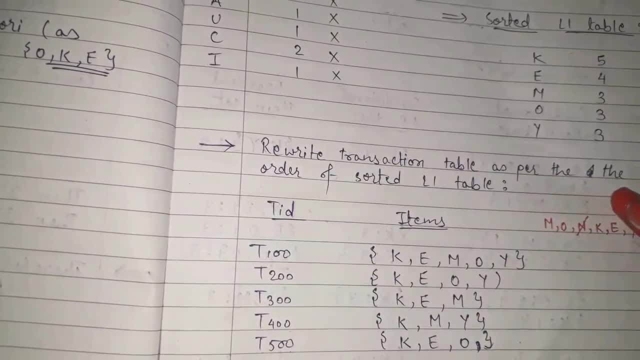 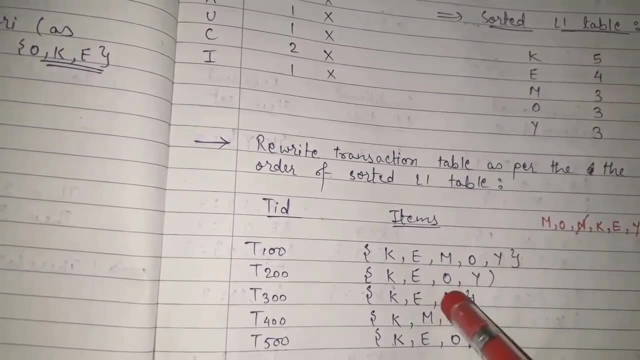 We will rewrite the transaction table as per the order of sorted L1 table. See this sorted L1 table is clear. We have sorted our L1 table. Then what we will do is These are the transaction IDs that are given to us: T100 to T500. 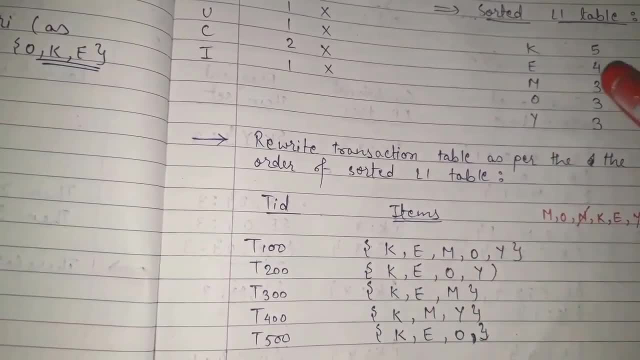 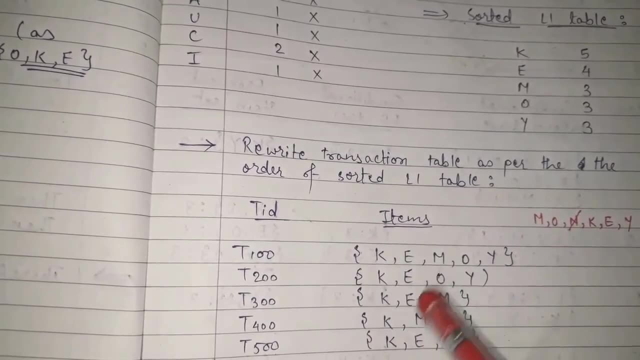 Now what we want to do is, As per the sorted L1 table, we want to sort the elements or the items of these transactions, only These transactions also. For example, see in T100 what we were having. we were having D6. M O N K E Y. 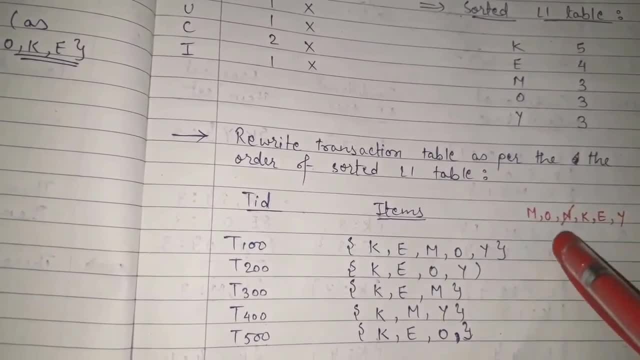 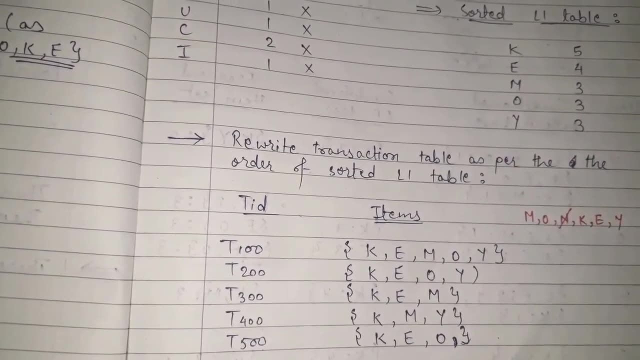 Fine, Now we want to do here 2 tasks. The first task is we have to remove the items that are not present in this table. That means that are having frequency count less than 3.. So see out of M O N K E Y N is not present in our L1 table. 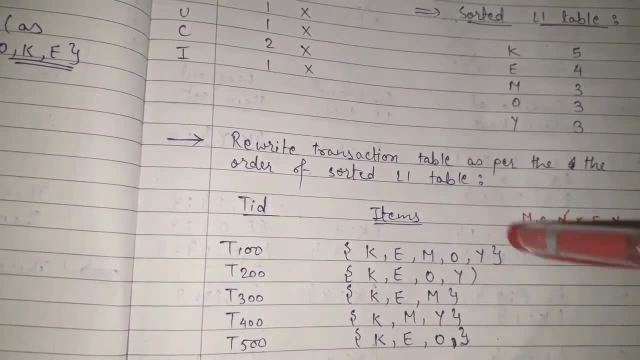 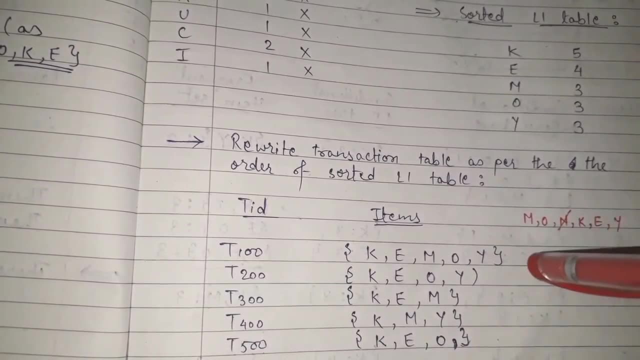 So, simply, we will remove N Means. whenever there is any item that is not present in L1 table, we have to simply remove them. So I have removed N. What are the remaining items? M O K E Y. So I just want to write M O K E Y here in this T100. 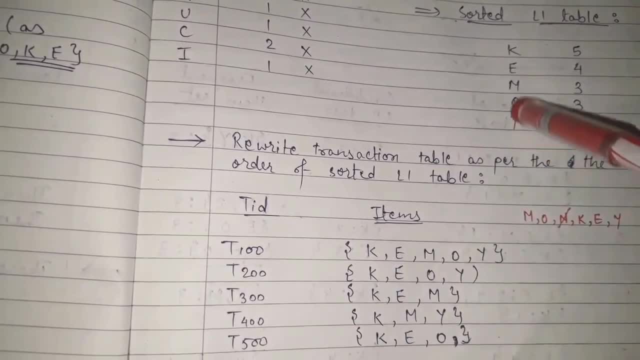 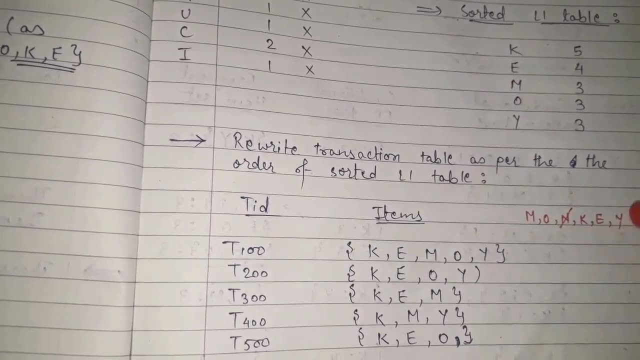 But that also how we will write. We will write it in This order only: K E M O Y, In this sorted order only. So instead of M O K E Y, I will write it as K E M O Y. Fine. 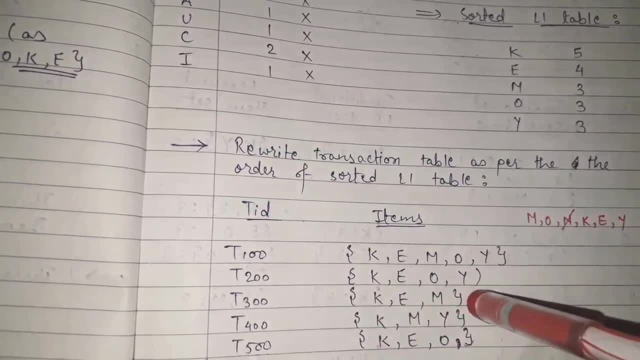 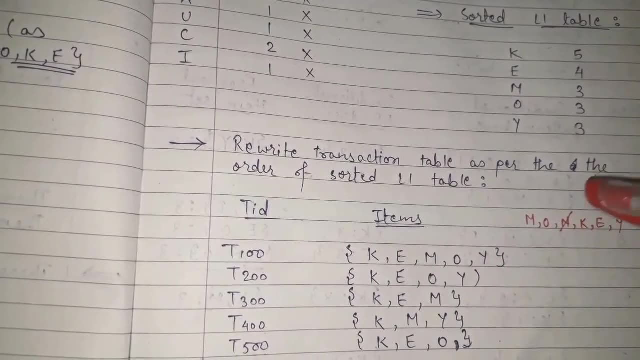 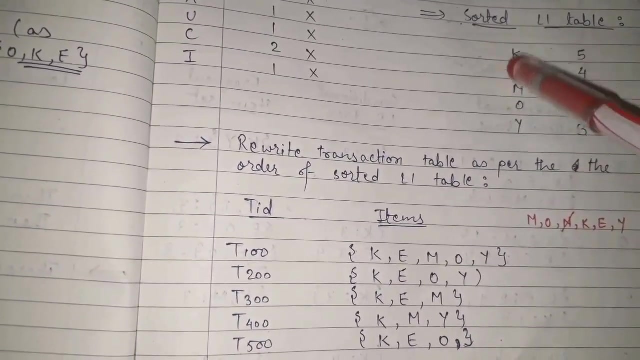 So I have written it like this. Similarly, in T200 we have done the same thing. We have removed the unwanted, or we have removed the items that are having frequency count support less than 3.. And whatever is remaining, we just have to sort them in this order. 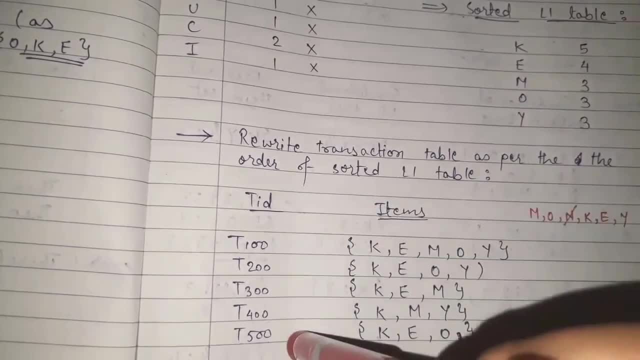 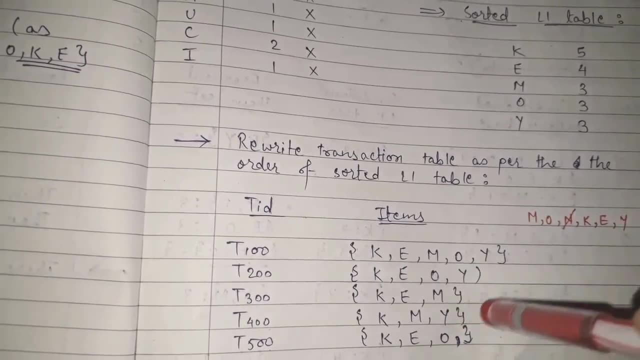 Fine, So in this way we will write the items for all the transactions. Got it? So this is again one important step. Simply what we have done. I hope you have got it. We have simply removed the items that are not there in L1 table. 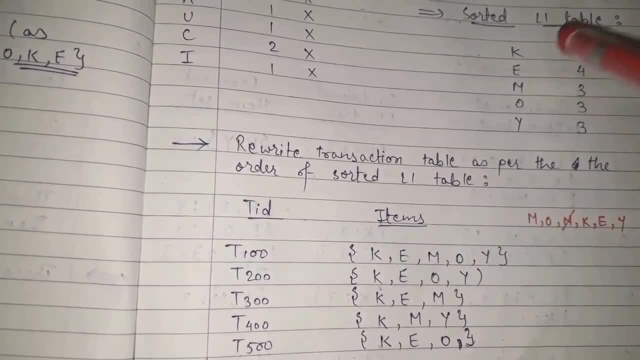 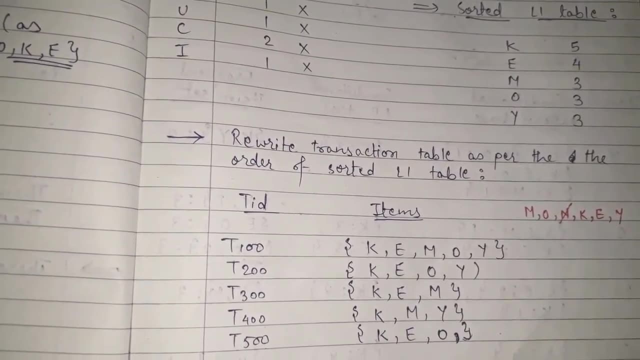 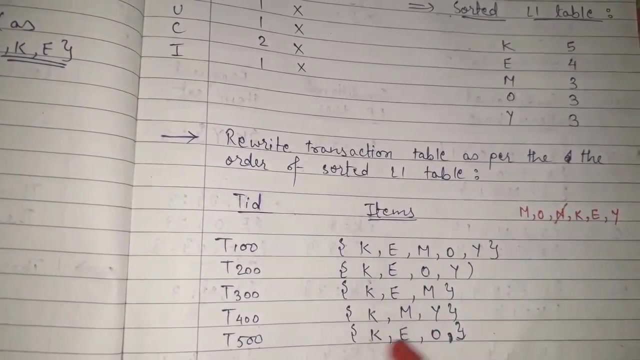 And for the remaining items, we have just arranged them in this sorted order. Fine, So we have got this. Now, after this, the main thing arrives, that is, how to make the FP tree. So once you are having this table ready with you Now, based on this table, we have to draw FP tree. 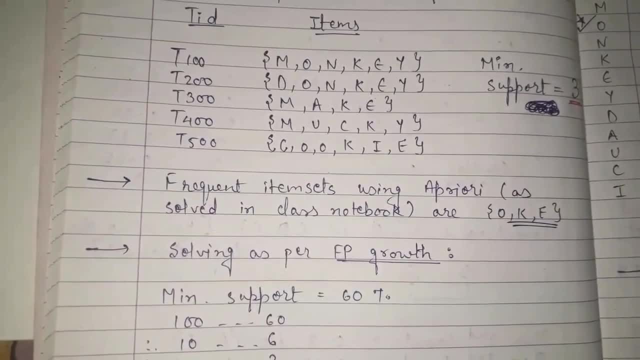 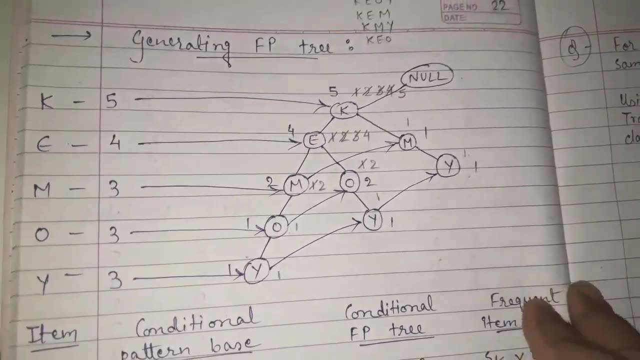 Now see this carefully, because making FP tree is one of the like, most important step in this case, And actually the problem is that many students are finding it difficult, But trust me, if you get the procedure, how to do it, you will not find it difficult at all. 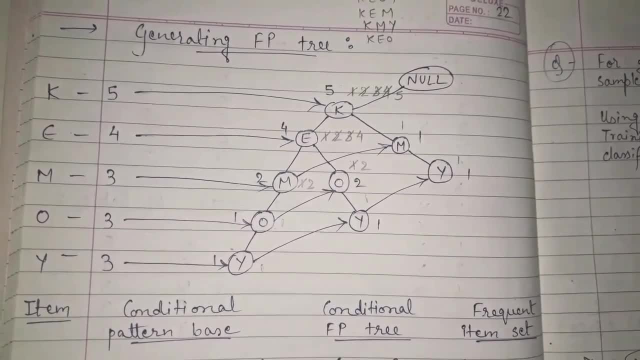 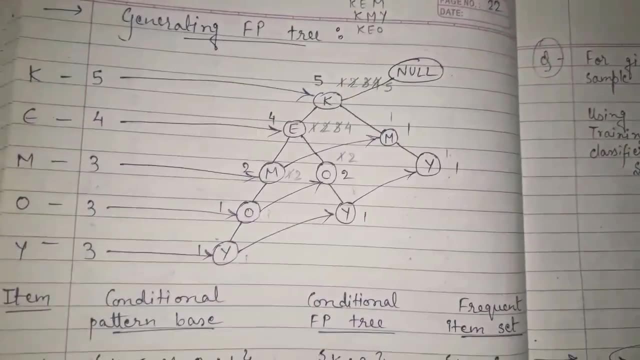 Fine, So let's see how to generate FP tree. It is simple. What we want to do here is We want to generate the FP tree. So let me tell you from the beginning: We are generating FP tree. What should be our first step in generating FP tree? 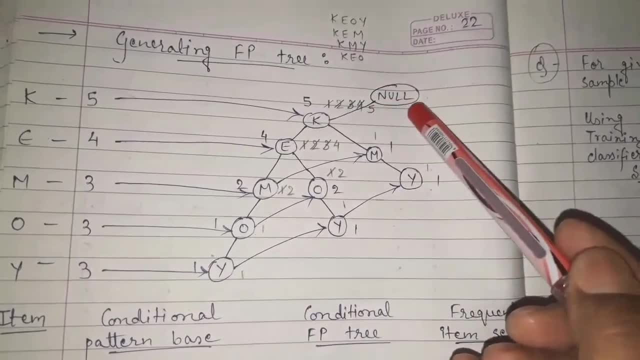 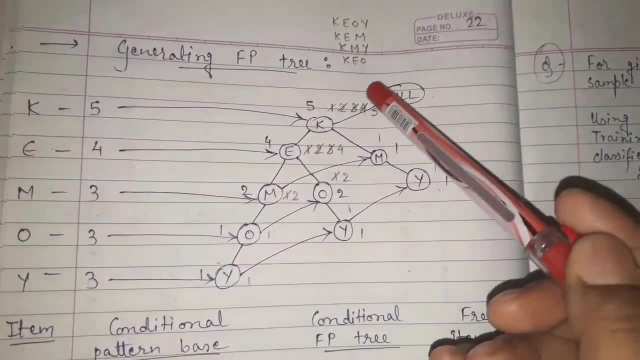 The first step is we have to draw our root node. In this case, our root node will be null. Fine, Remember this thing: that for generating FP tree, our root node will always be null. So the first step is we will write null here in the beginning. 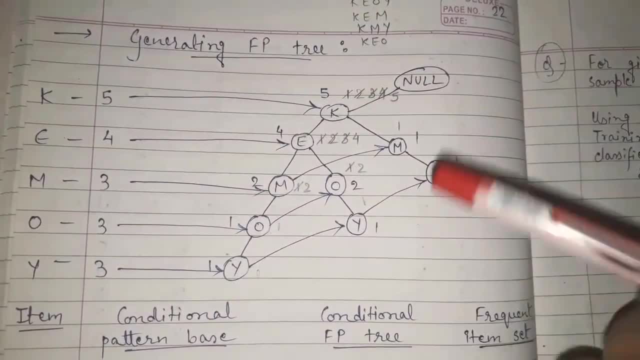 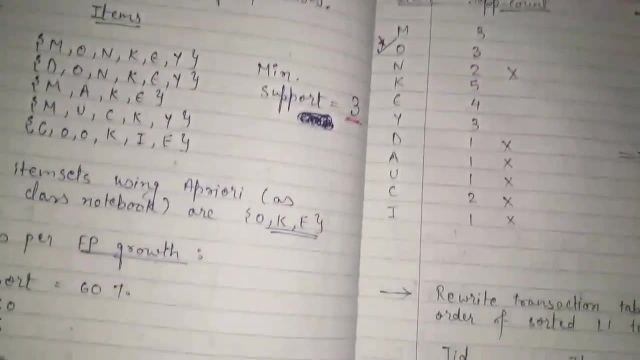 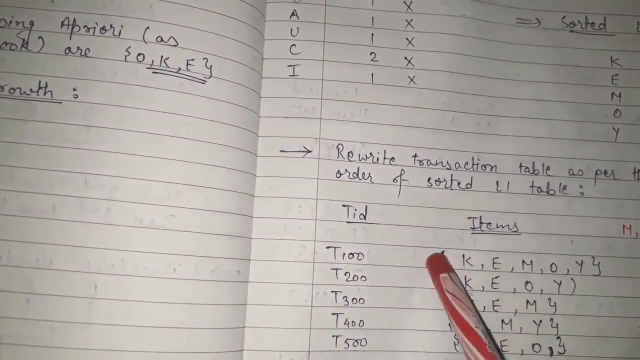 And then we will start to begin. Then we will begin to add our nodes. Now, After drawing null, what you need to do is you need to consistently check your table, Whatever table you were having, Fine, So, simply, what we need to do is, one by one, for each row, we will add the items in our tree. 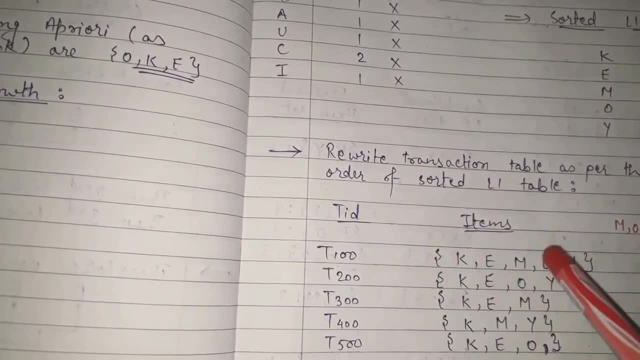 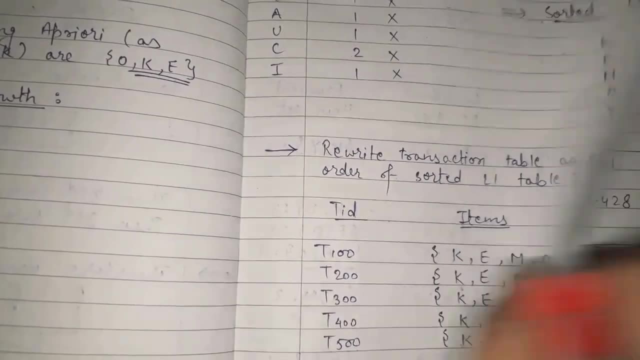 So for the first row, or for the first transaction, what our item set was KEMOY, Fine, KEMOY. So I just see KEMOY and then remaining four. I have written it there So we can directly see. 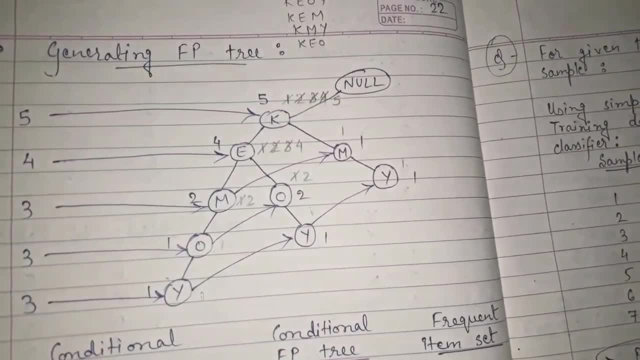 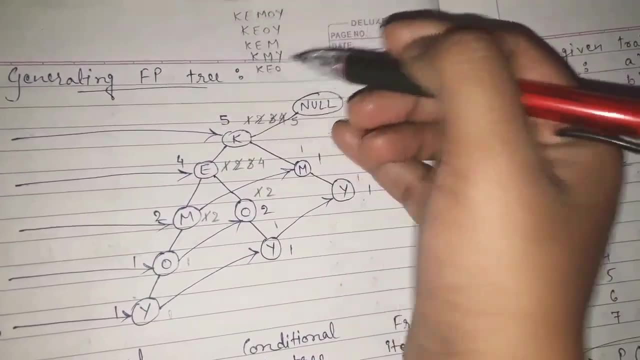 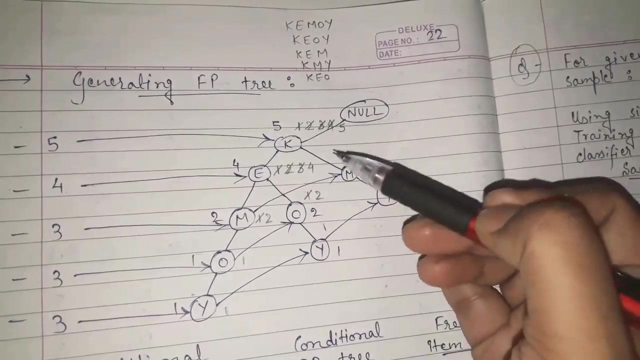 See these four, and the first one was KEMOY. These are the five items for our five transactions. Fine, So the first thing is KEMOY. So what I will do with null? I will simply add this: KEMOY. 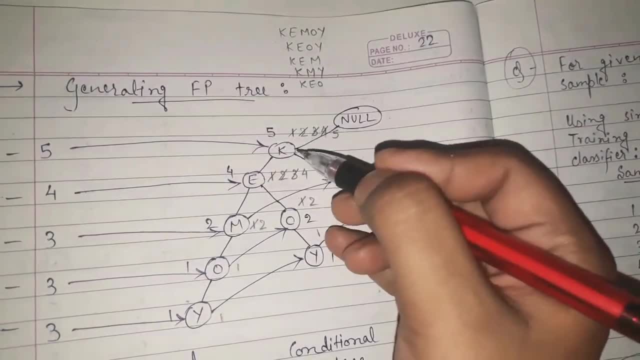 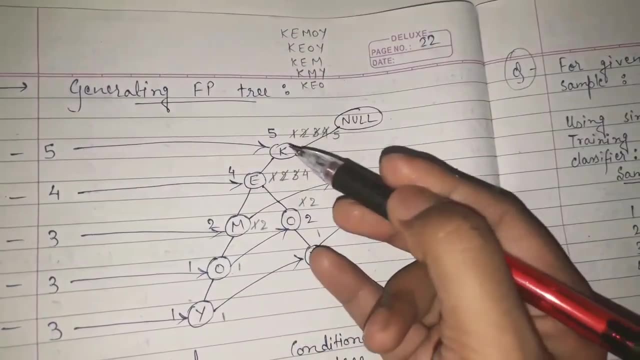 Okay, So see What will happen: that whenever I am writing this KEMOY for the first time, I will assign the weight one for them. Fine, As you can see here, I will assign one for them Then. second is KEOY. 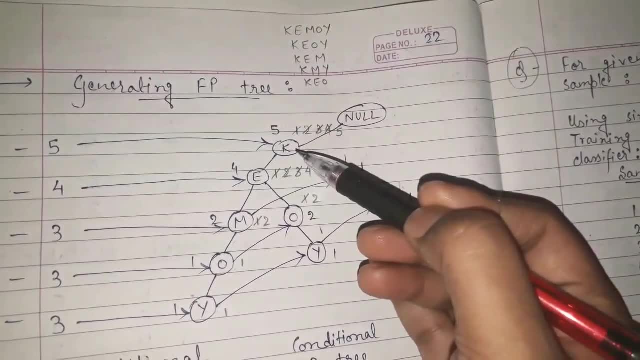 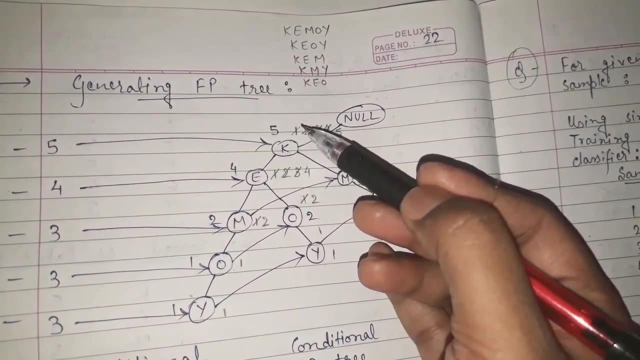 Now, if I start with null, K is already available. Yes, So I don't need to add K again. I will simply increase this counter and I will remove this one and make it two. I will increase this counter by one, Fine. 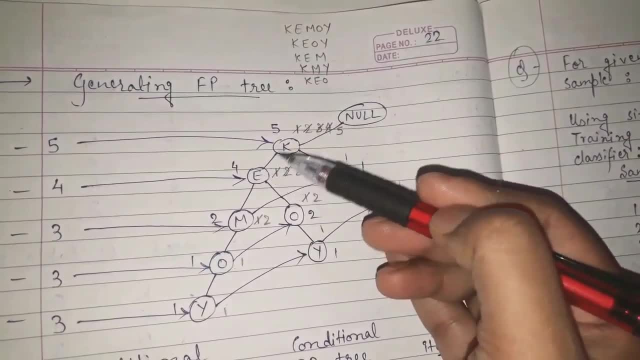 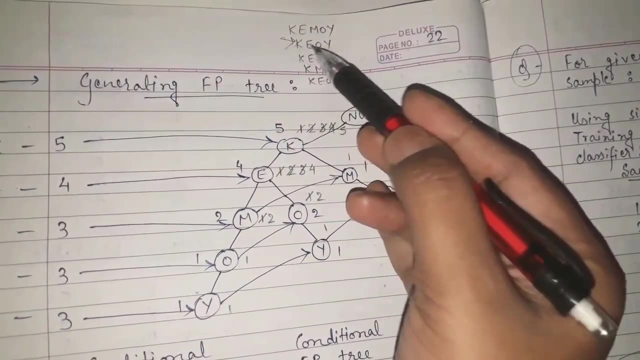 So KEOY, Now after K E, is also available, because we have added this whole thing, KEMOY, We have added this whole thing. So in the second step, what we want is KEOY, So after K E is also available. 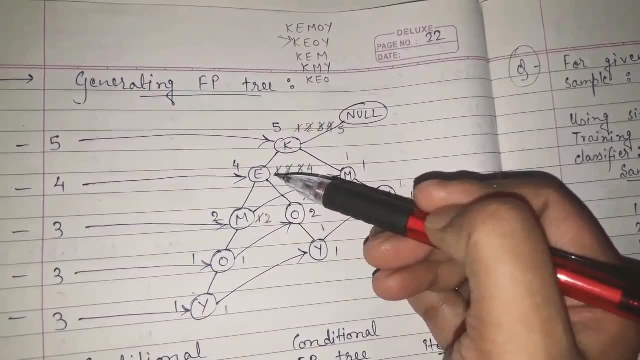 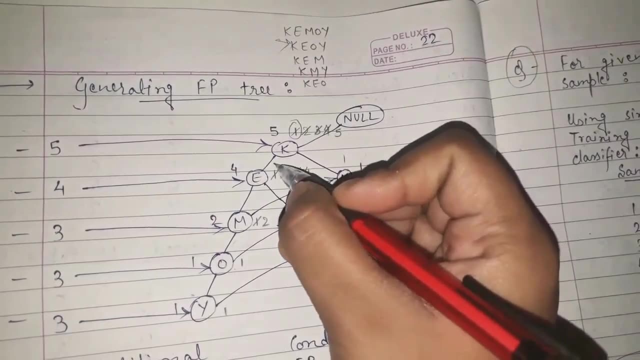 Yes, So I know I don't need to add E again. I will simply increase the counter for this also. So see: here also, we have cancelled out one and we have written two. Here also, we will cancel out one and we will write two. 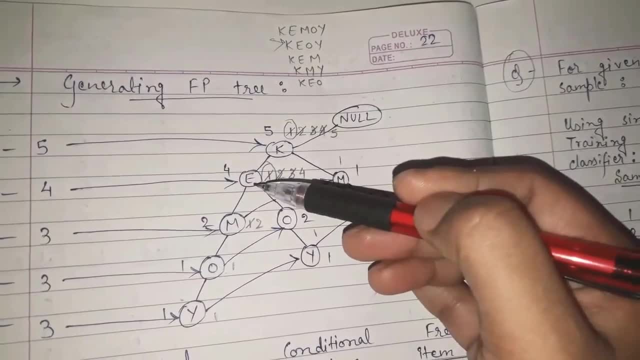 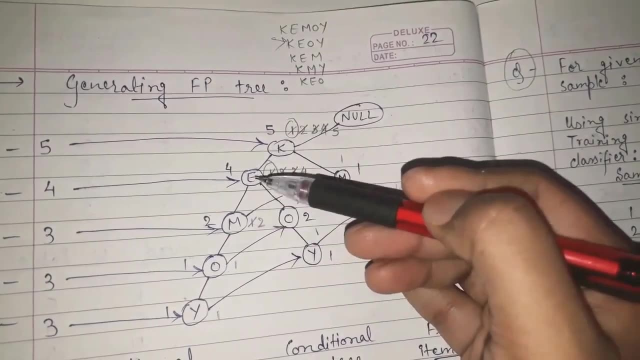 Fine, Okay, KE, then O. Now, after I, after E. if I check, am I having O? No, So what I need to do is O is not already present after E, So after E, I will add one branch for O. So after E, I will add this branch for O. 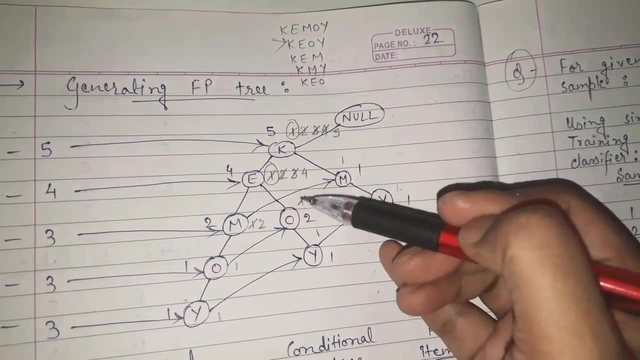 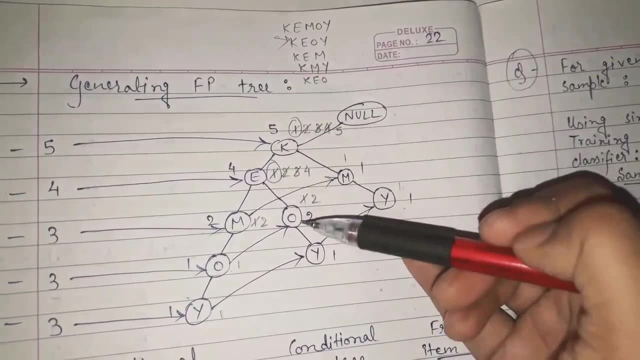 Got it. So I will add this branch for O and I will write one here because I am adding it for the first time. So I will write one here. Then, after O, I want Y, After O nothing is there, So I will add Y, because O I have added recently. 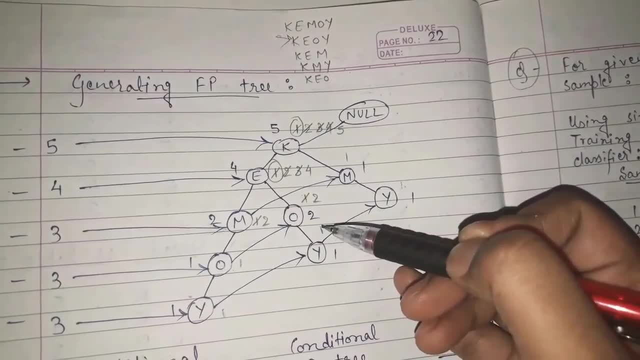 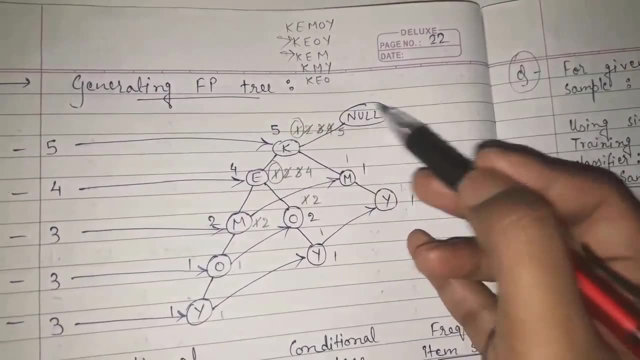 So I will add one node of Y and I will write the counter for Y as one. Fine, Okay, Then we are having KEM Now from NULL. if I start K, K is already there. So what I will do? I will simply increase the counter. 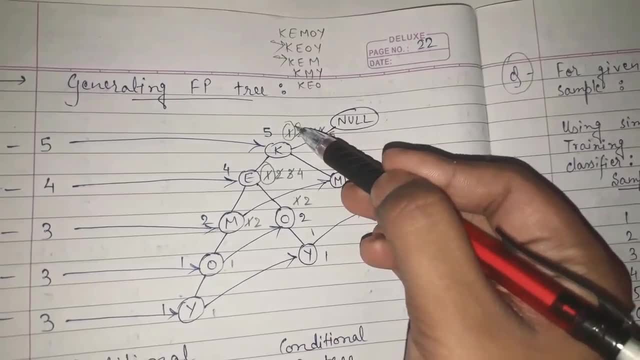 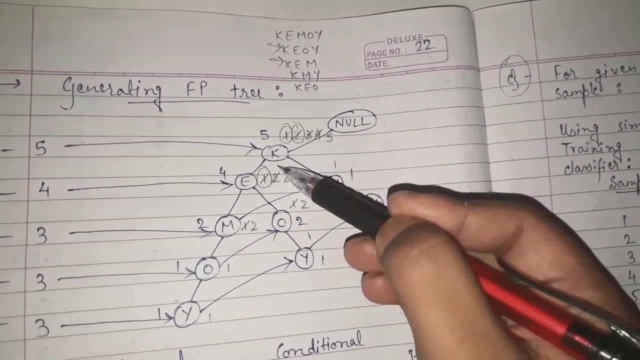 One, two, Now two was there. Now. I will cancel out this two and I will write three here. KEM After K. I am having E, Yes, So I will increase the counter from two to three. I will cancel out two and I will write three. 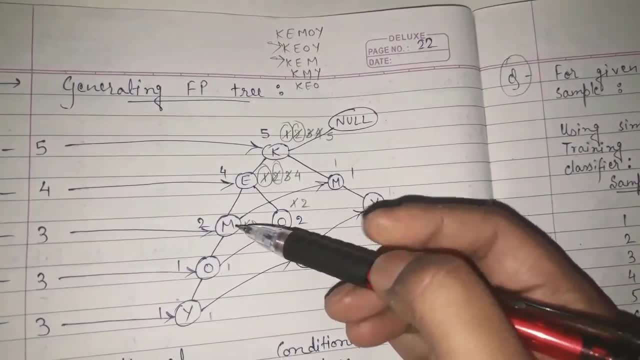 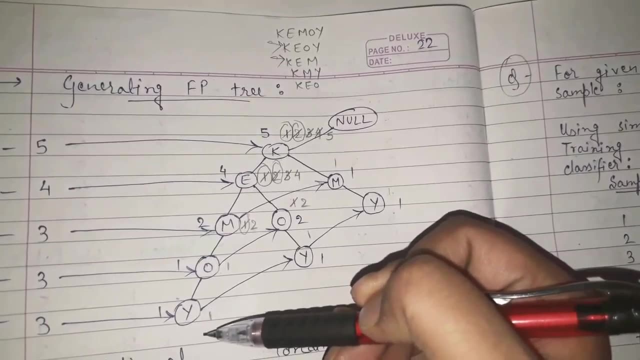 KEM Now after E M is also available. Yes, So now I will cancel out one and I will write two here. Whatever nodes are already present, we do not need to again add it. We will simply increase its counter. Fine. 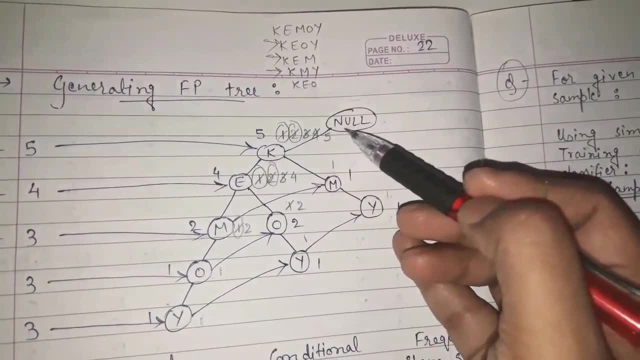 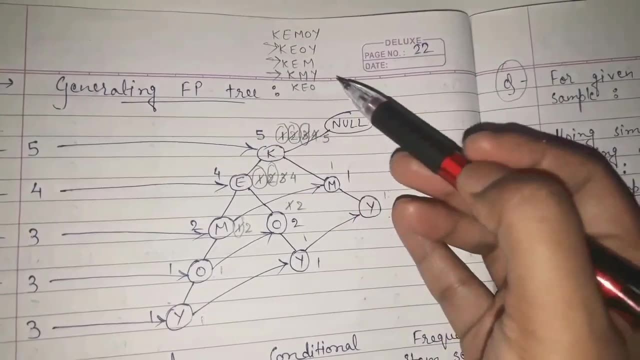 So KEM is also done. Then we are having KMY Now. initially K is available. Yes, So we will increase the counter from three to four, We will cancel out three and we will write it as four KMY Now after K M. 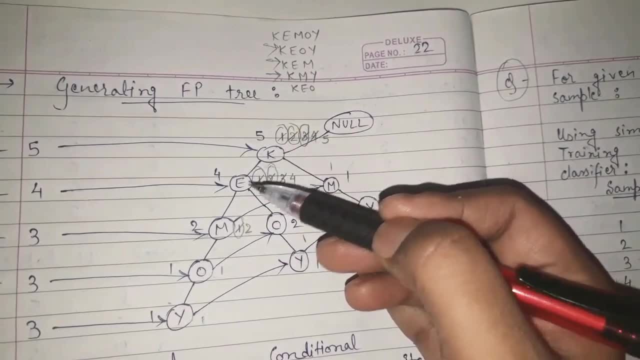 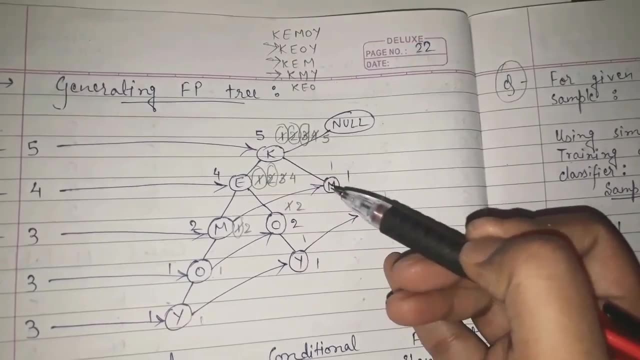 M is available. No, After: K E is available, but M is not available. So what we will do, We will make the branch for M. So we will make the branch for M, and M is arriving for the first time, So I will write the counter as one. 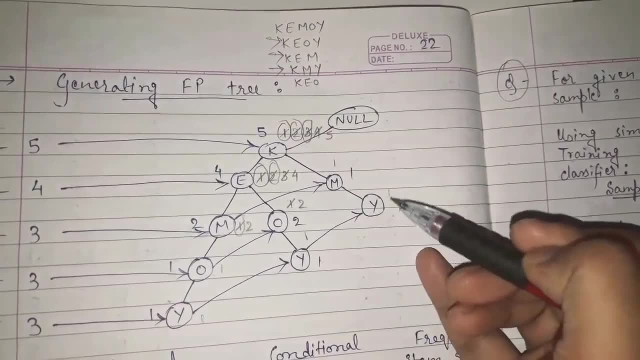 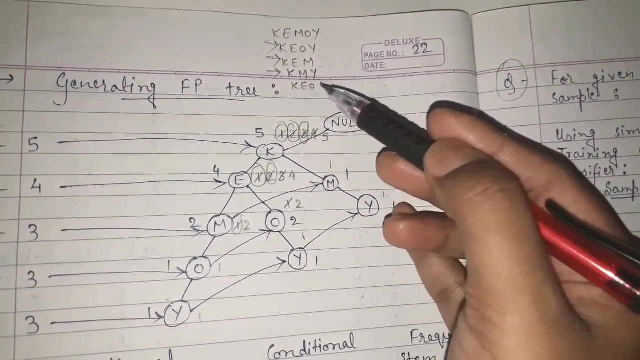 KMY. Then after M I have to add Y, also with the counter one. Then I am having at the end- Yes, At the end I am having KEO. So K is already there. So I will increase the pointer from four to five EO. 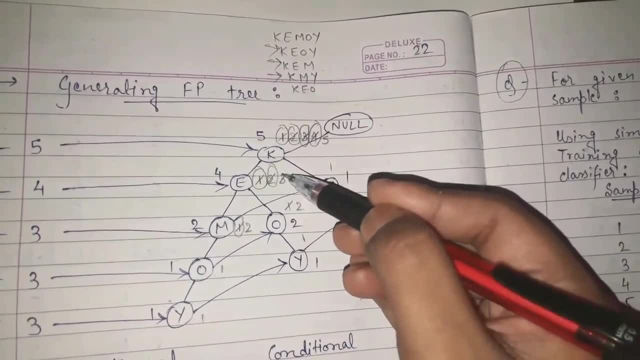 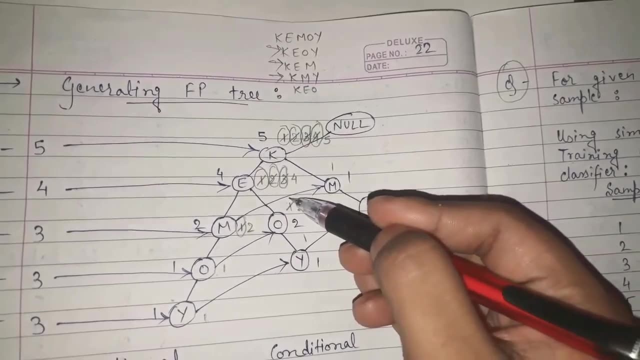 After K: I am having E, So I will increase the counter from three to four. Then I am having O. Yes, O is also already there, So I will cancel out one and increase the counter to two. Fine, all the item sets we have added in our tree. 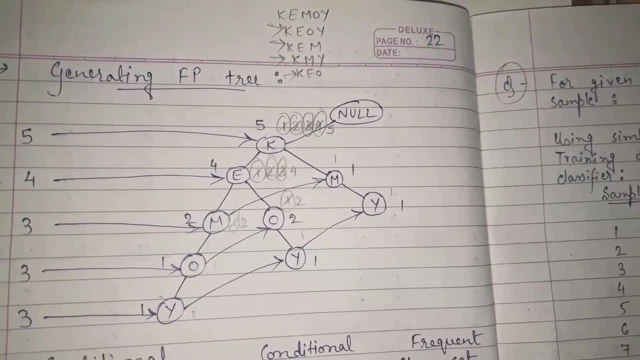 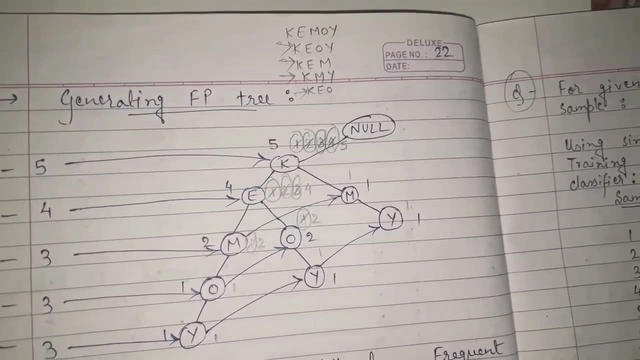 So our task is done. Now, how can we check that our task is done properly or not? So if you check your L1 table- existing L1 table, See sorted L1 table- If you check your sorted L1 table, you will find that it is done. 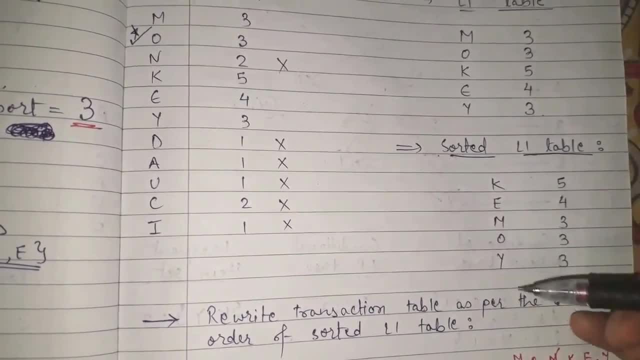 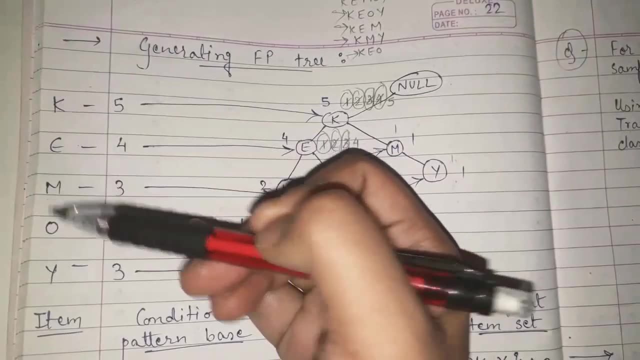 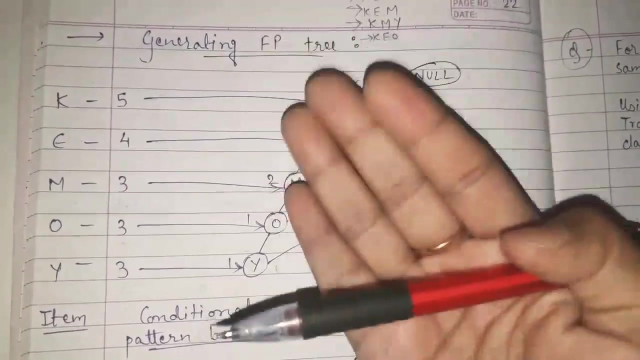 your sorted l1 table you have the value of kemoy, that is 5, 4, 3, 3, 3. fine, kemoy, just write it down: kemoy: 5, 4, 3, 3, 3, fine. so this is the data you are already having in our sorted l1 table. now what we? 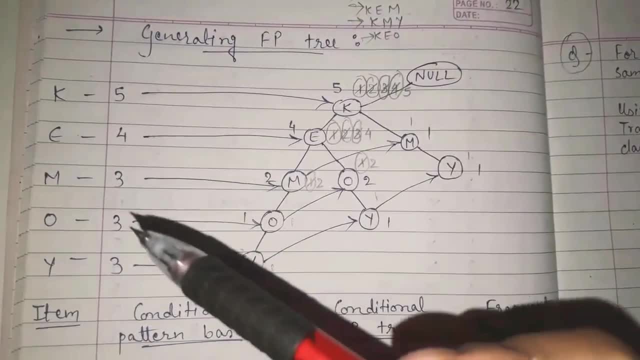 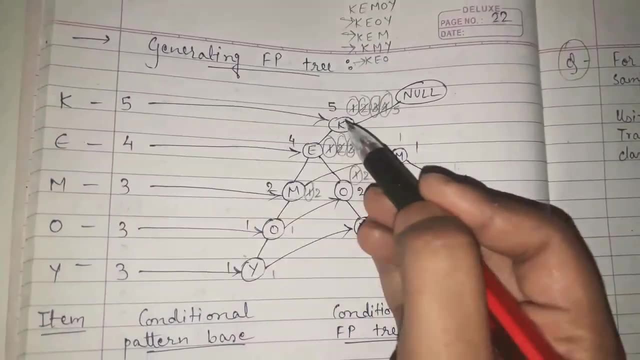 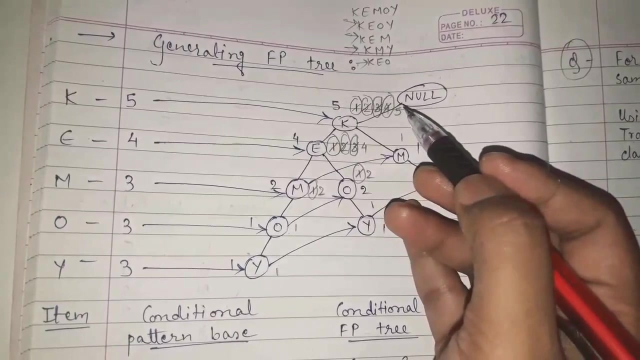 need to do is, after generating this fp3, just try to match these numbers that are, your frequency counts. are matching or not? so if we talk about this k, this k node, what is the current weight of k 5? fine, we have updated the counter 4 times and ultimately we are having the k value as 5. so yes, 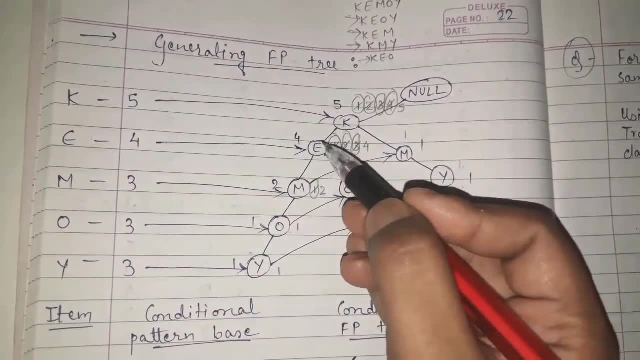 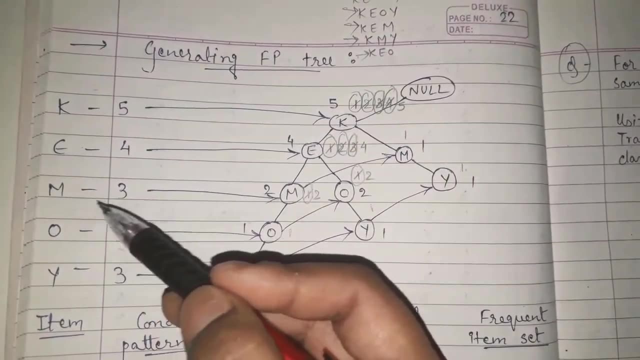 it is being matched. so we are correct. e is 4, so the current value of e is also 4. so yes, just match it out. and e value is 4. that is also correct. now. m is 3 in our table. m is 3 now if we talk here. 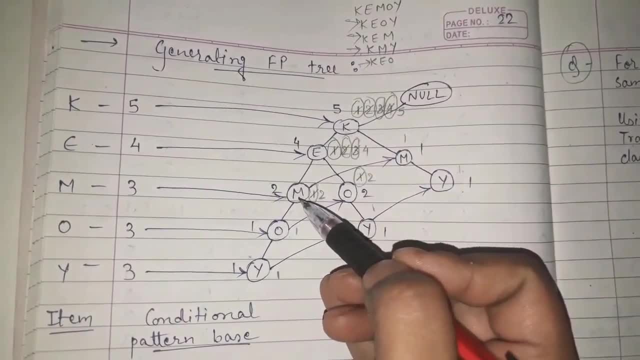 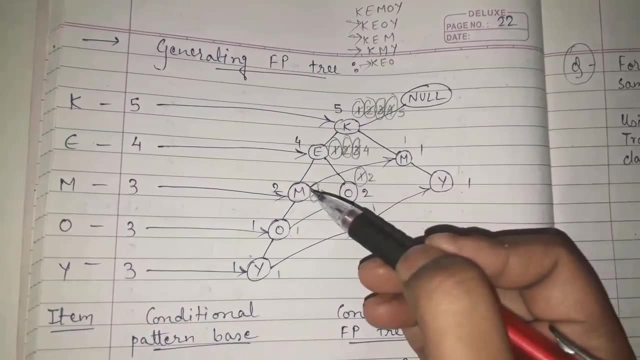 if we see here: here the current counter of m is 2. any other m is there? yes, one more m is there, having the current counter value as 1. so just connect this m with that m. here the value was 2, so 2 plus 1 is 3. 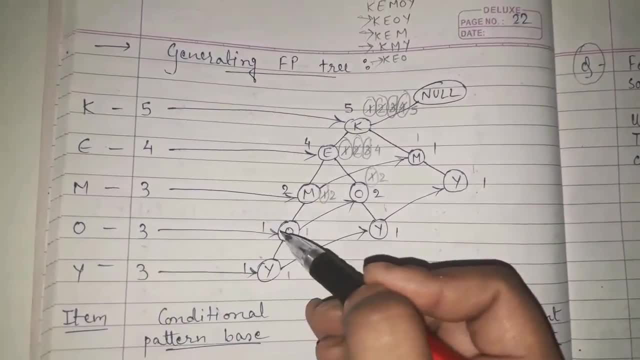 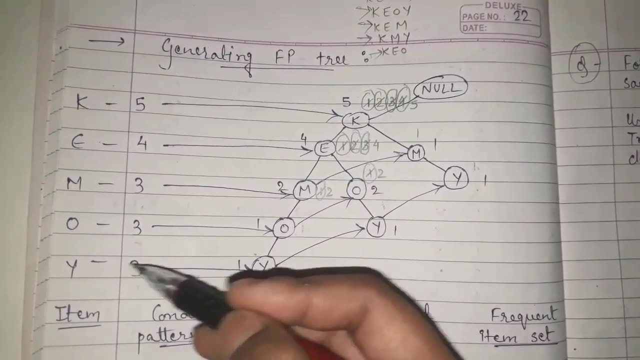 so our 3 is verified, fine. similarly o. here the value of o is 1. connected with this o, the value is 2, 2 plus 1 is 3. then if we verify this y, here we are having y as 1, another y as 1. 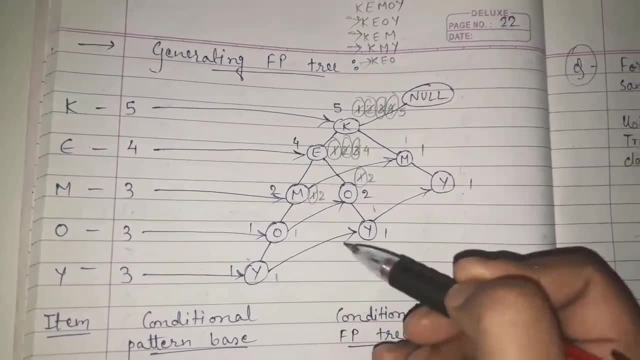 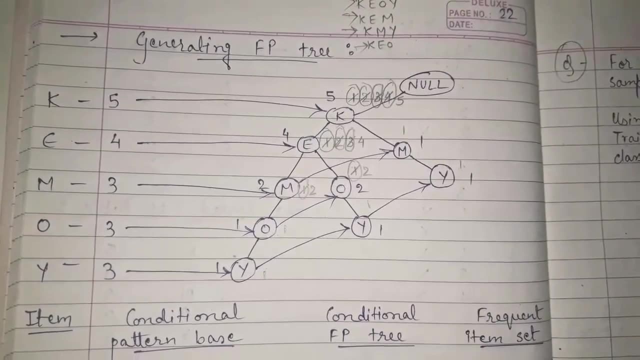 connected with another y as 1. those y are there with 1- 1- 1 value. so ultimately, 1 plus 1 plus 1 equal to 3. this y equal to 3 is verified, fine. so this is the most important task here to generate. 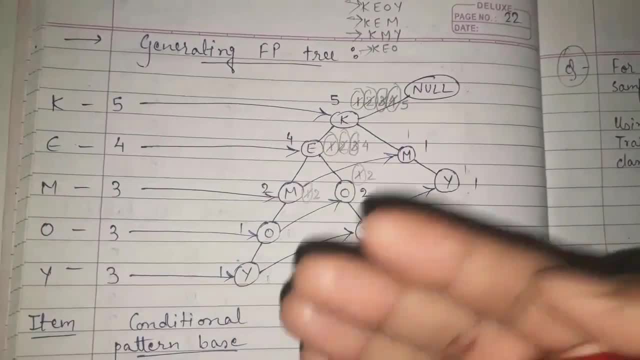 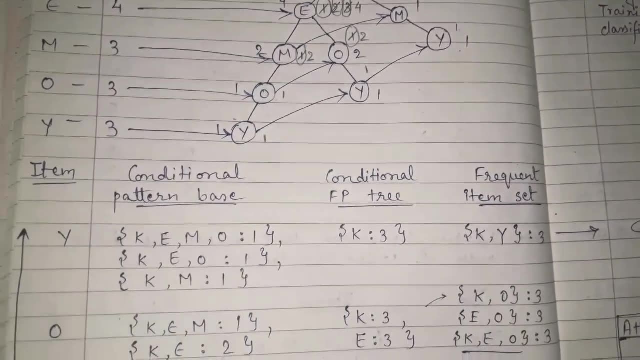 the Fp3. hope you understood it properly. now, once your fptree is generated properly, now the last task is you have to make a table to based on your FP tree, and now see the table which are the fields of your table. item: conditional pattern types. now, after generating, we are getting the number which it. is and that the number one factor- it is the function fp has- is the tiles, the columns that you will be generating. what are the tiles? guess? I am running the whole table now and because the table is in all the value, okay, so click you will see we have the function create the table name and groups all of these tables. 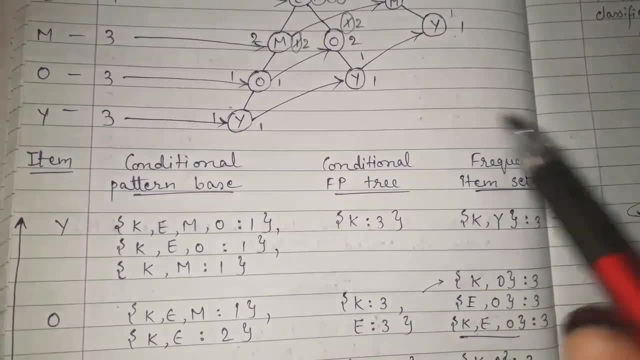 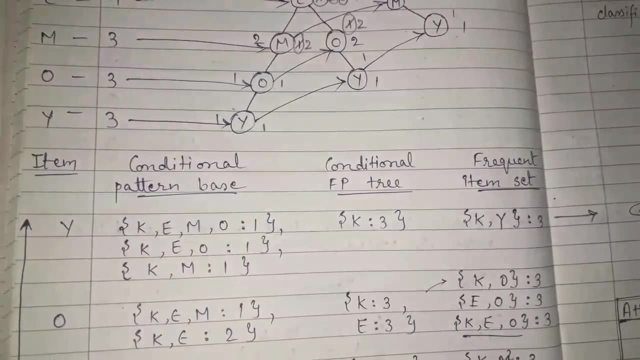 let us see for our table, which are the functions and what are the jóvenes going through. so let us measure pretty conditional pattern, base, conditional FP tree and frequent item set. Now let's check. let me tell you one by one, field wise that how we are filling the table. 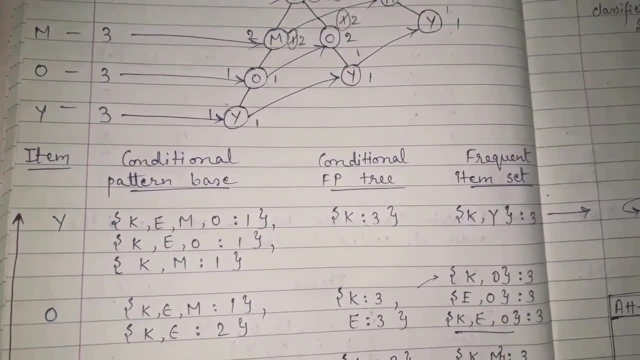 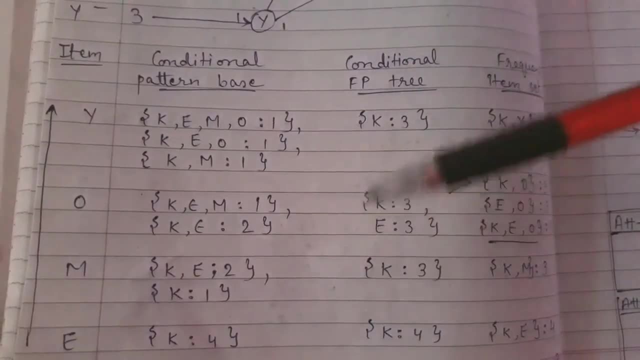 Once you got this, after this table, we will directly get our frequent item pattern. fine, So first of all, let's see how to take the items. fine, So, simultaneously, you have to see your FP tree and, based on that, you have to fill the values. 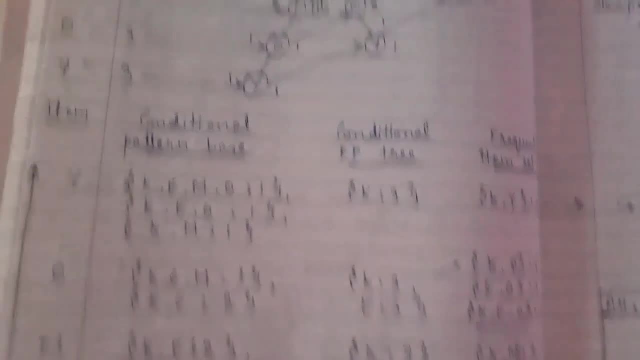 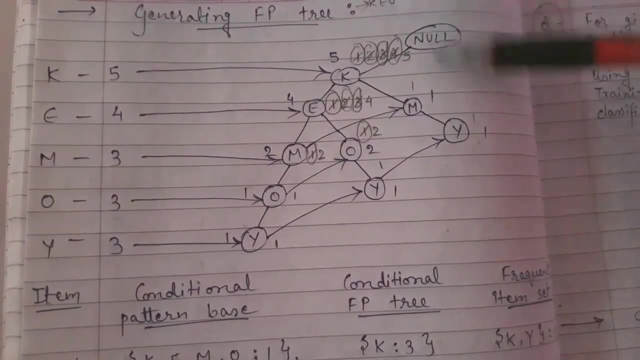 So, first of all, if we see how we will fill up this, items is see in the tree. this is the null, this is the default null node that we have written, So we don't need to consider that. apart from that, whatever nodes we are having, 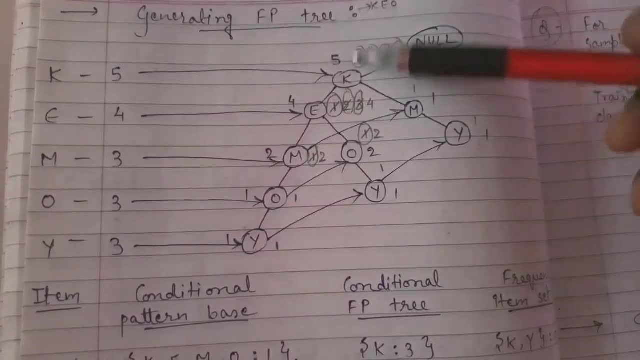 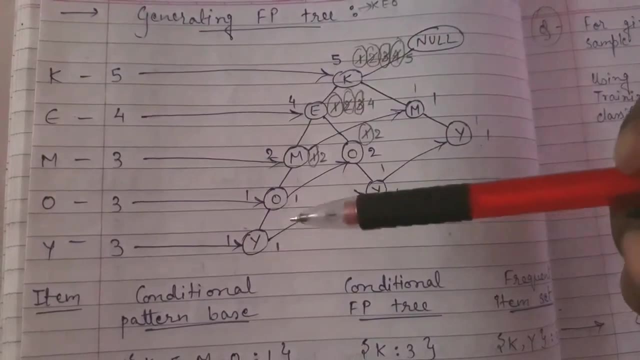 In this also this k, say this k is our highest node, this is our root node. fine, So we don't need to write this k. also, apart from k, whatever remaining nodes are there from the bottom, we have to write it. So if we see from the bottom, we are having y o. 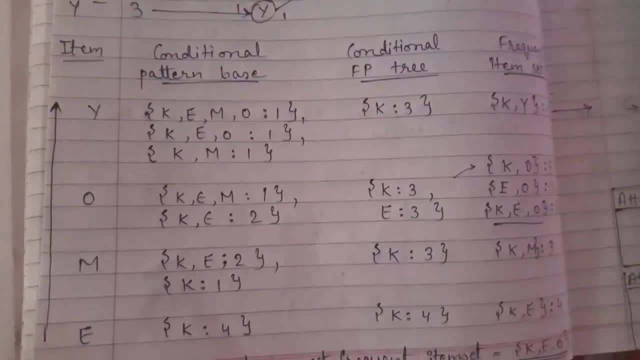 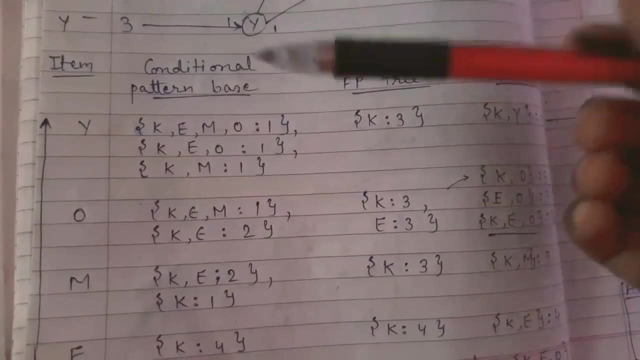 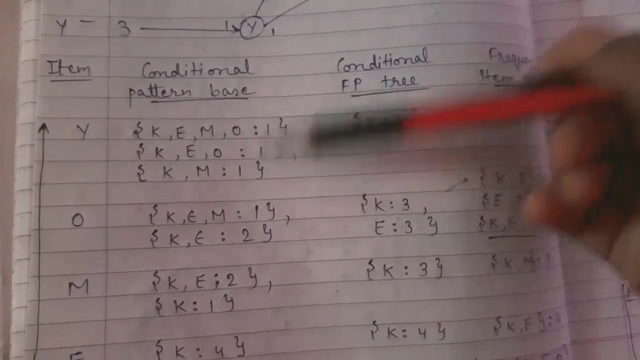 m e. So we will write y o m e in the item field y o m e. fine, So this will be our item. now comes conditional pattern base. Now, what we will write in the conditional pattern base is that, whatever our item is how we are reaching up to this item, what is the path see? first of all, we are having y. 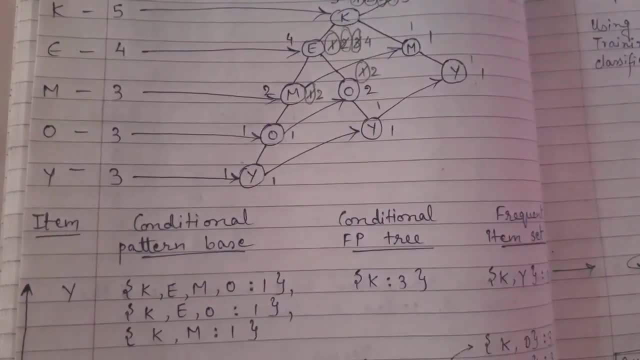 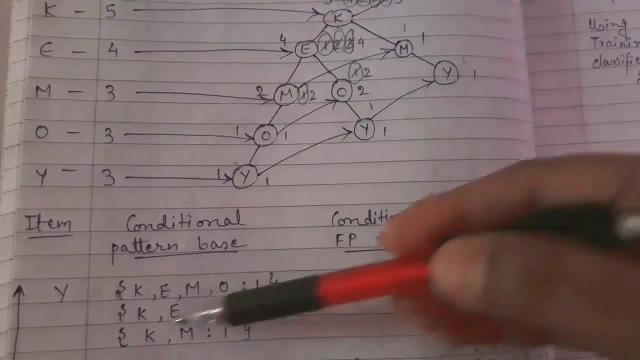 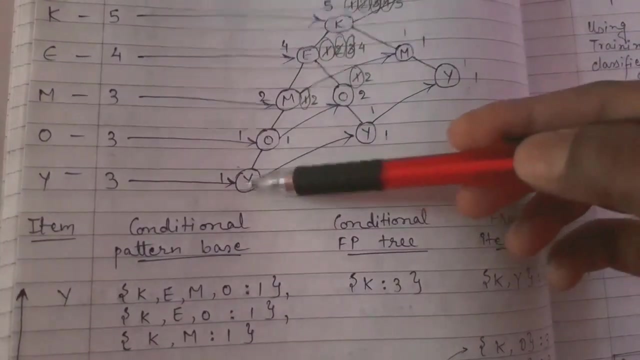 So if we see here how we are reaching up to y, see we are reaching up to y through k e m o, fine. One way is k e m o. so we have written k e m o and after colon what we are writing, that after coming from k e m o, the weight of y is one. so this is one, and again we are having 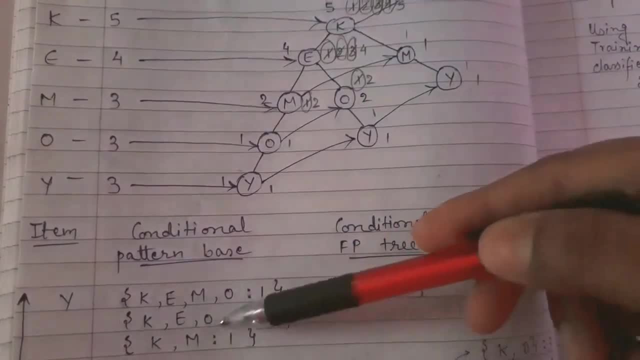 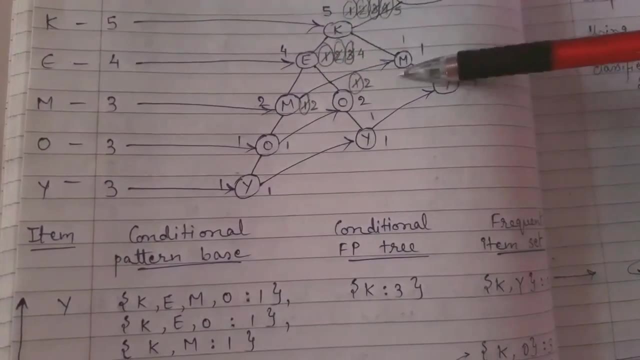 one more y how we can reach here k e o, So k e o, colon one, because its weight is also one. then we are having y how we are reaching to this y k m through k m and the weight is one, so k m, colon one, simple, fine. 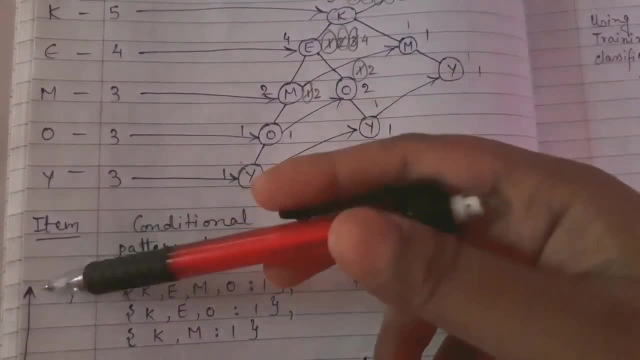 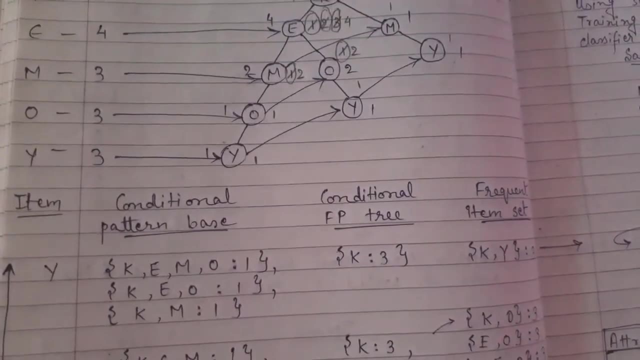 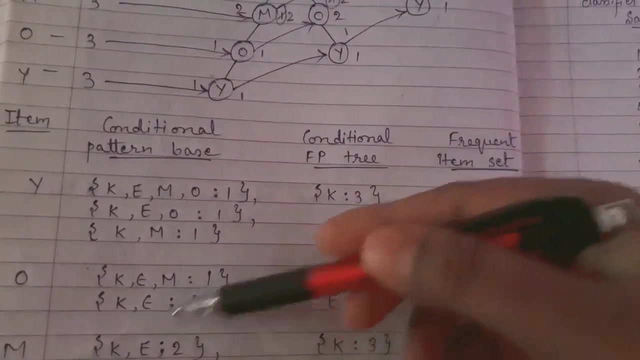 So in this conditional pattern base We just have to write that how we can reach up to this item. and similarly, let me show you one more o we are having o. so see here we are having o, how we are reaching this o k e m and the weight is one. so k e m colon one. k e m colon one. any other o is there? yes, 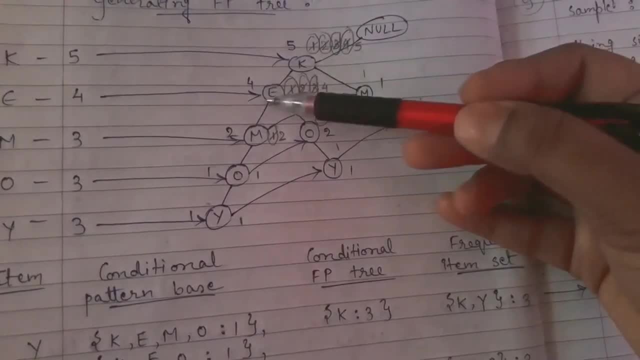 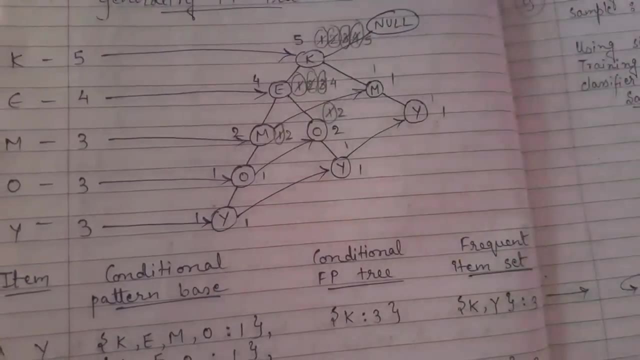 again. here also we are having o how we can reach here. k e colon weight is two, so k e. we have to write this ultimate weight, fine, So the ultimate weight is two k e colon one, k e colon two. so the next one is k e colon two. fine, so similarly for all the item sets. 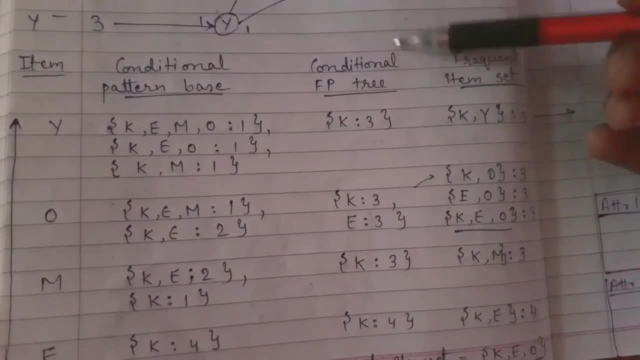 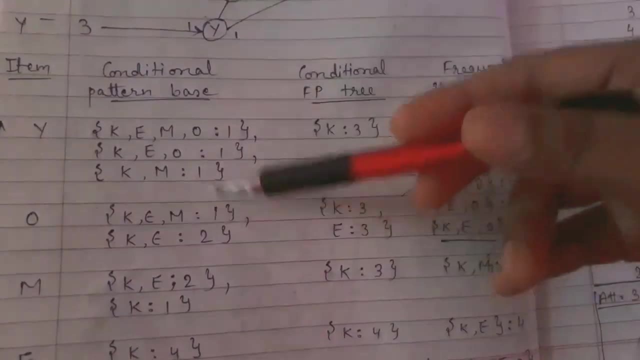 we have to write the conditional pattern base. fine. then we are having conditional fp tree. what do we write in this conditional fp tree? we will write this: the value of this field based on the value of this field. fine. so how we can do that, see conditional in conditional. 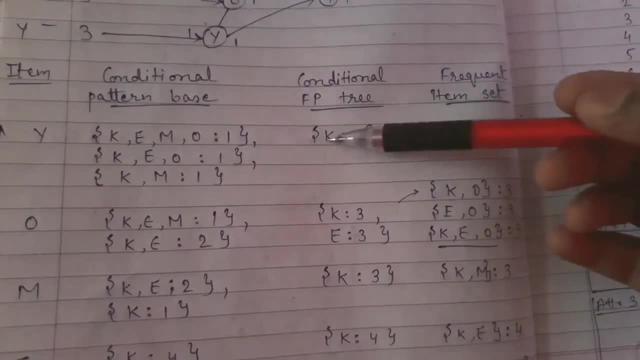 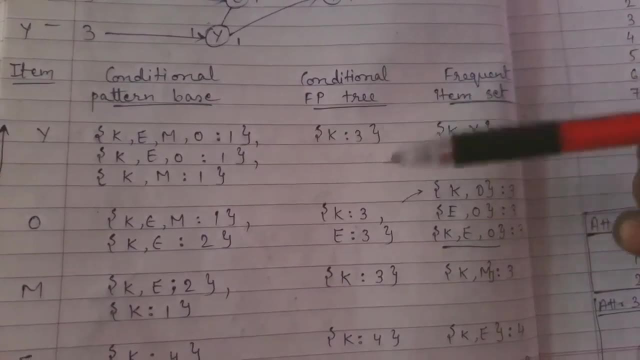 fp tree. we just have to write the count along with the item that is occurring at least three times. Because we were having minimum support count in our question, minimum support count is given as three, so whatever item is repeating at least three times, we have to write it there. 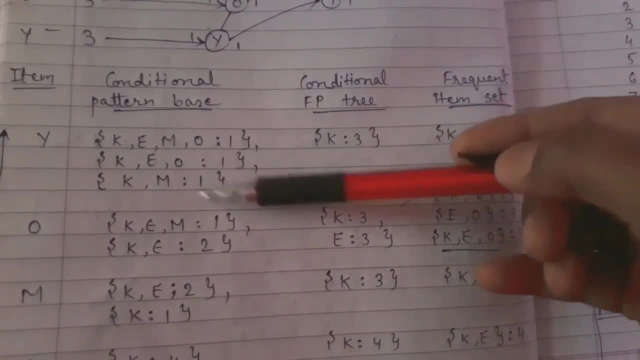 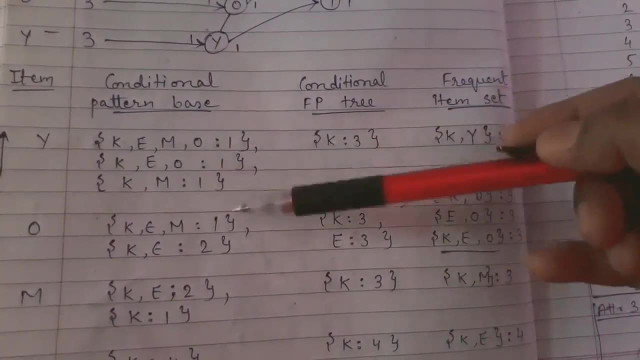 see we are having k thrice and the weight is one one one, so k is occurring three times, one plus one plus one, so k, colon three. there is no more item which is repeating three or more than three times, so we will write only this: in this case, k is repeating two times. 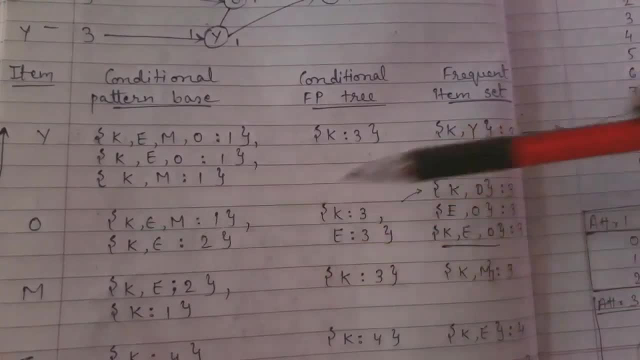 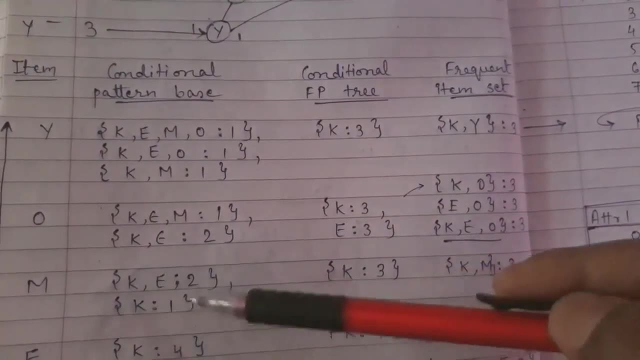 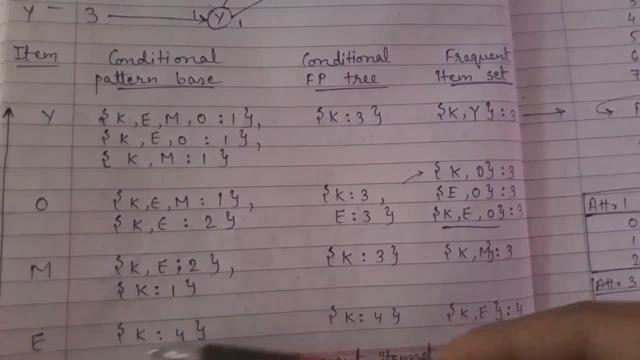 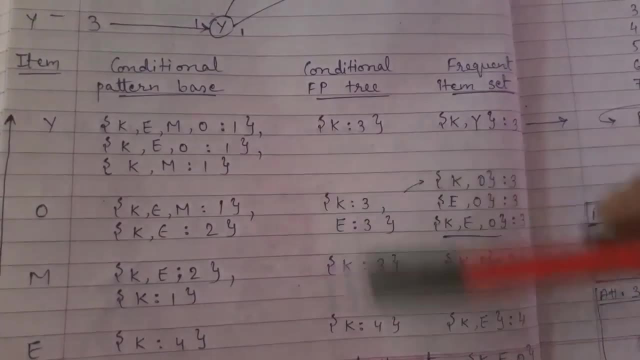 the weight two, so it is less than three. we will not write that again here. k having weight four, that is greater than three. so we will write k with the weight four. so in the conditional fp tree we will write it like this. then at the end we are having frequent item set in. 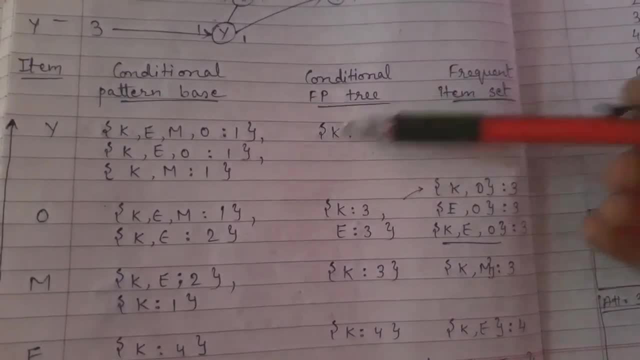 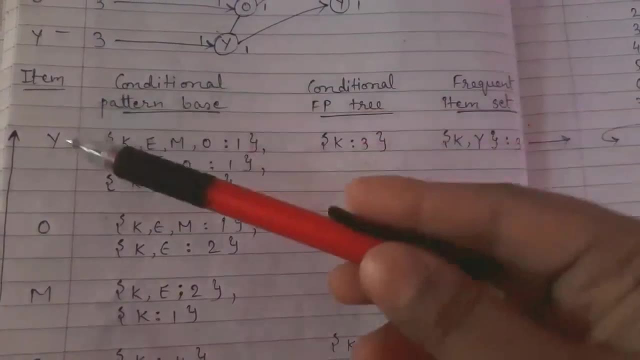 the frequent item set. we do not need to do anything, But whatever is present in our conditional fp tree we will combine it with the item and we will write it here. Here we are having k for the item y, so k, comma y, colon three. so this is our one frequent. 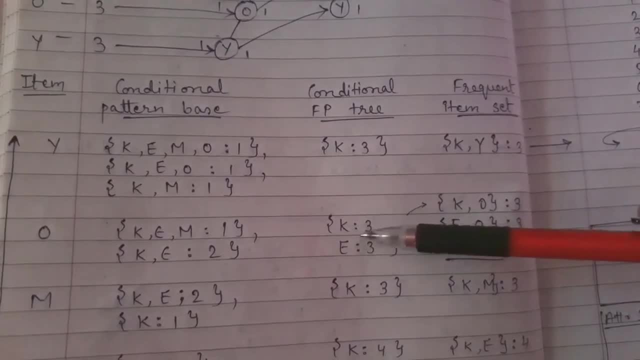 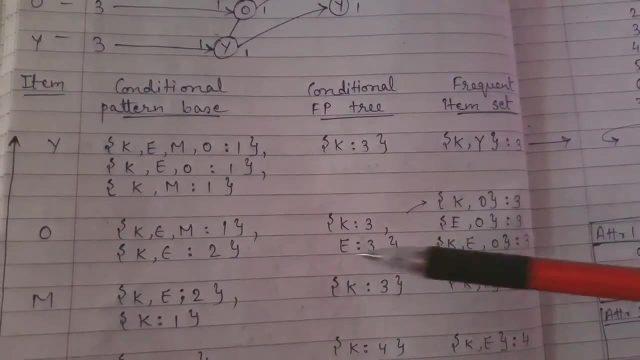 item set. here we are having k e- two items. so what we will do, we will combine them with o, individually and also together. so one pair will be k o, one pair will be e o and one pair will be k e- o together, and all the weights will be three. 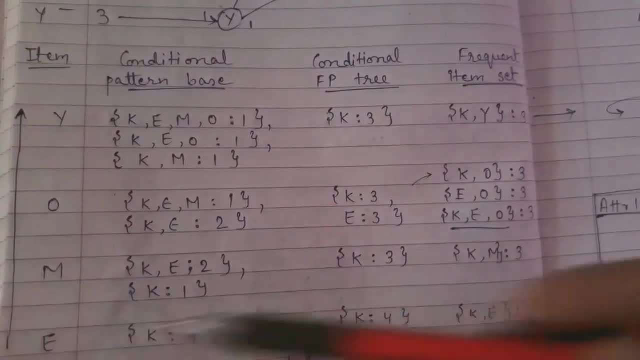 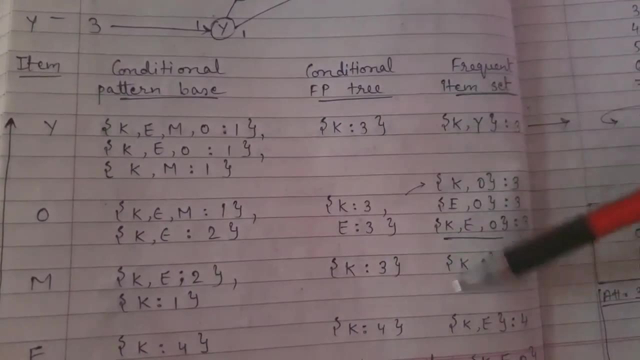 Similarly, k m having the weight three and k e having the weight four. fine, so in this way we can make this whole table now at the end of the table. these are the frequent item sets that we got, but, as in the question, we know that we want to find out the most frequent. 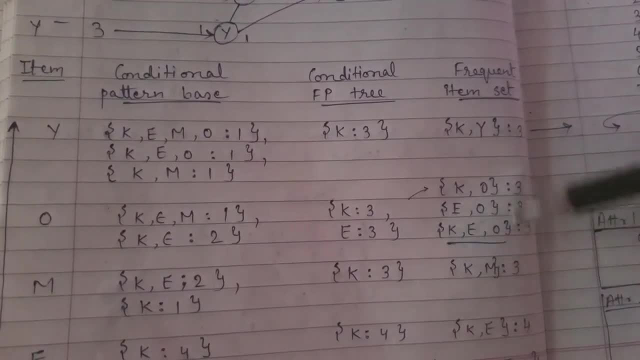 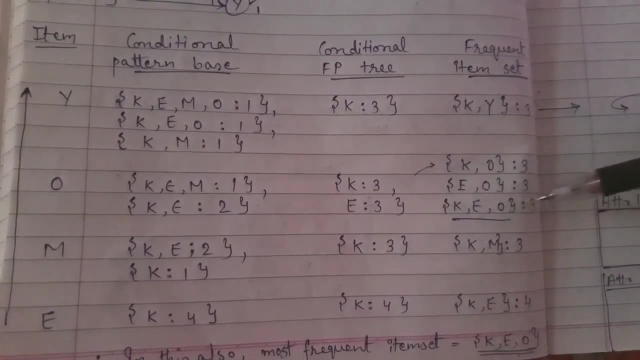 set having three items. so here we know all the item sets are having two items. this is the only item set having three item sets, that is, k e o having the weight three. so in a priority we know that we got k e o and k e o having the weight three. 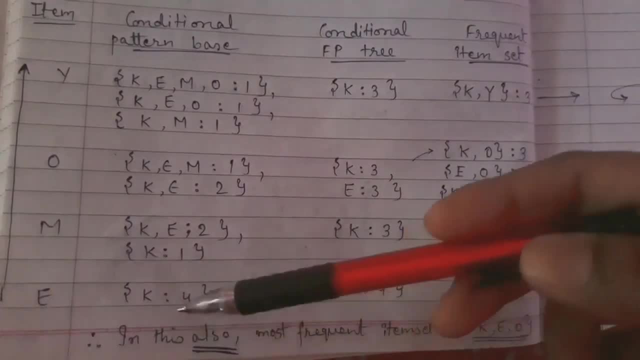 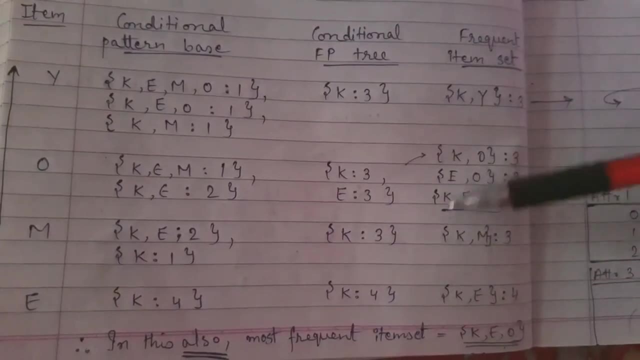 So here we got this item set, only k e o, and here also in this fp tree also the most frequent item set that we got is k e o. fine, so in both the methods k e o is the most frequent item set that we got. I hope you have understood the whole procedure. you have understood the. 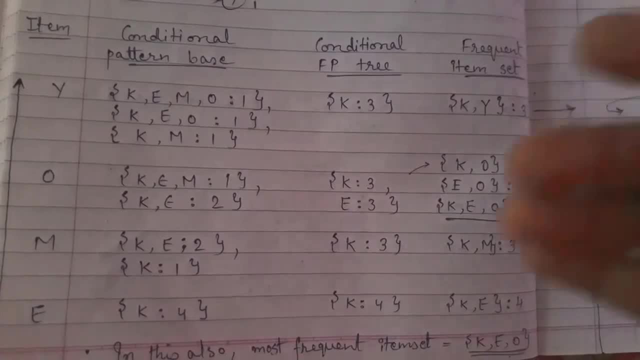 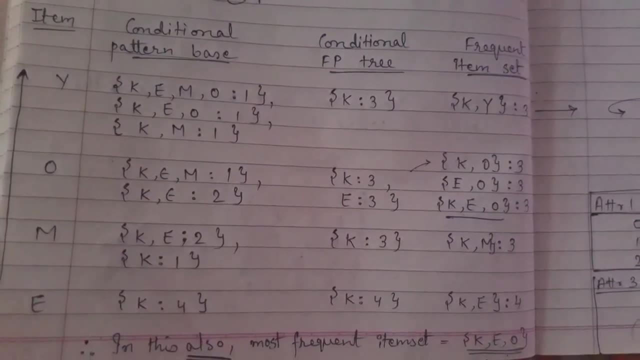 whole all the steps. once you practice couple of examples, you will get the thoroughly clear idea of how to solve it out. fine, if you like the video, if you found it helpful, please, please, like it down. please share it with more and more people and I will see you in the next. 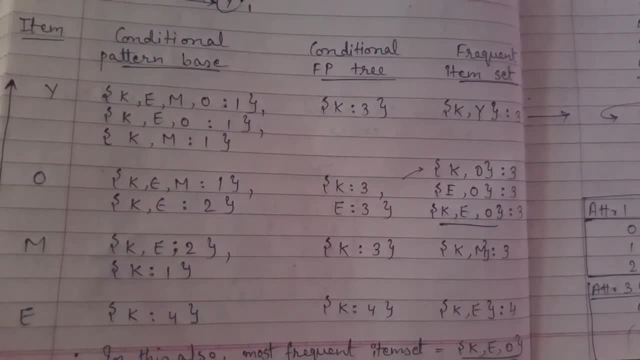 video. If you have not subscribed the channel yet, please subscribe the channel. thank you so much.